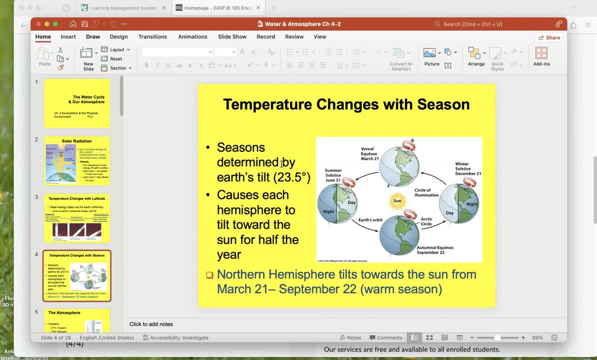 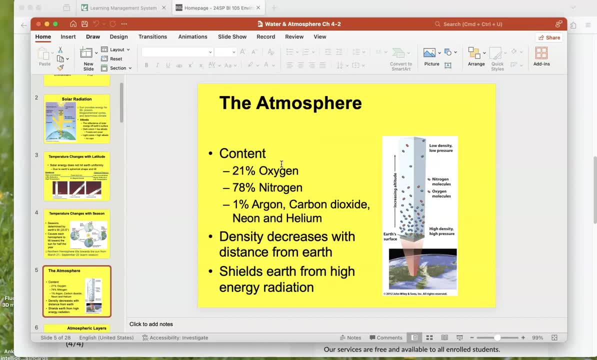 So that's the main reason, And it just keeps bouncing back and forth. We could also spend a little bit of test questions, maybe on the composition of the atmosphere. Okay, Fairly straightforward stuff: A little bit of oxygen, a whole lot of nitrogen. 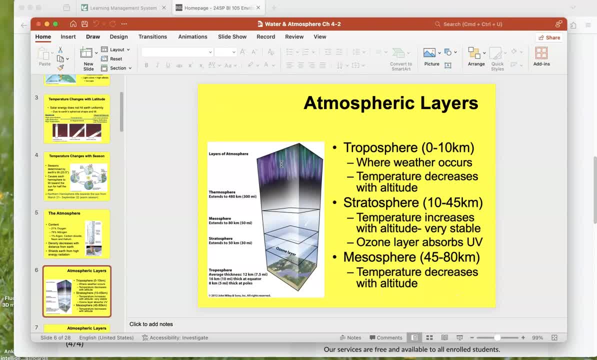 Remember we had our levels. You guys live in the troposphere. All right, This diagram, you know this word goes with the bottom. Unfortunately, these are kind of little arrows pointing, But so you guys live in the troposphere. Above us is the stratosphere. 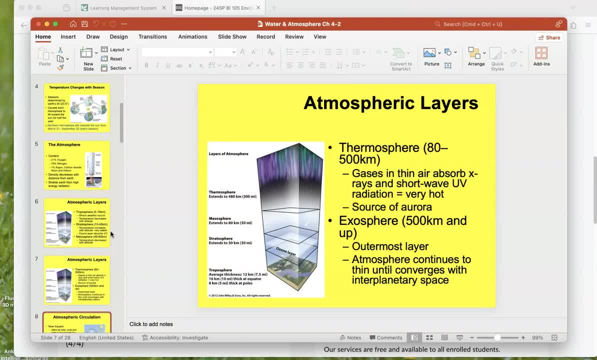 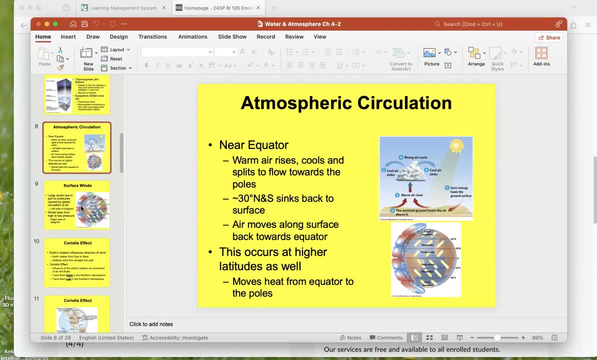 And then exosphere we move up to, That's, outer space. All right, Let's not, unless you guys have spent tons of time already learning your upper atmospheric circulation patterns. Have we? Have we? Well, maybe you'll be able to put it to use later in life. All right, All right. 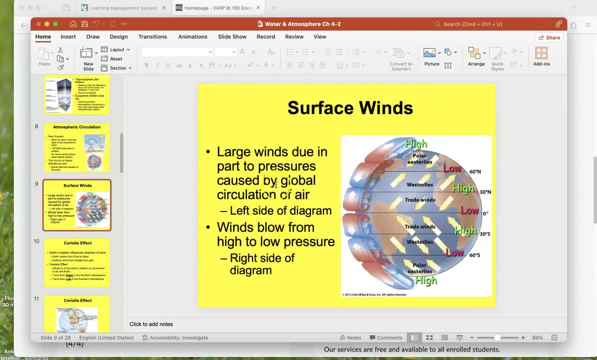 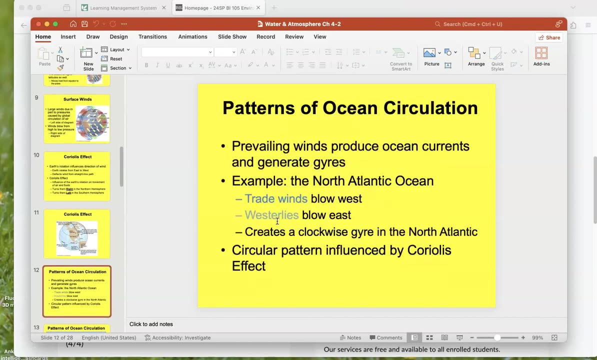 So let's, let's not worry too much about these. They are, you know, kind of cool to know what the trade winds are in the westerlies and so on and so forth. But we will skip that for this semester. Coriolis, I'm not going to even touch. 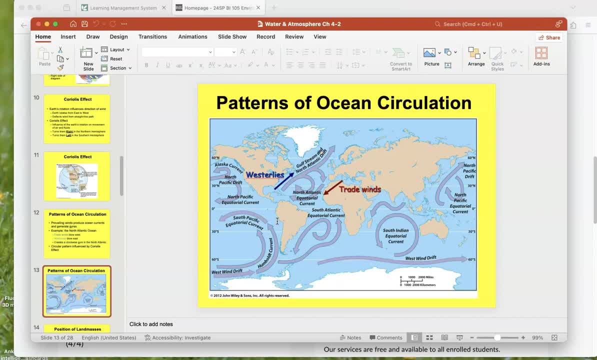 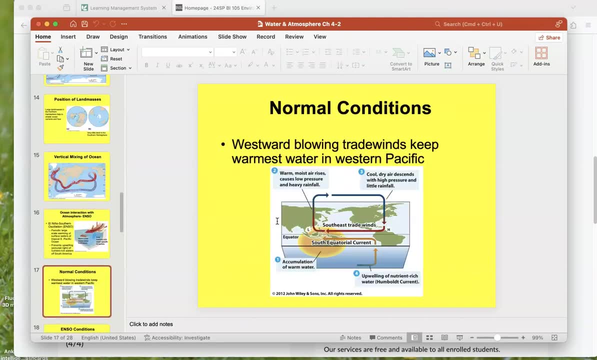 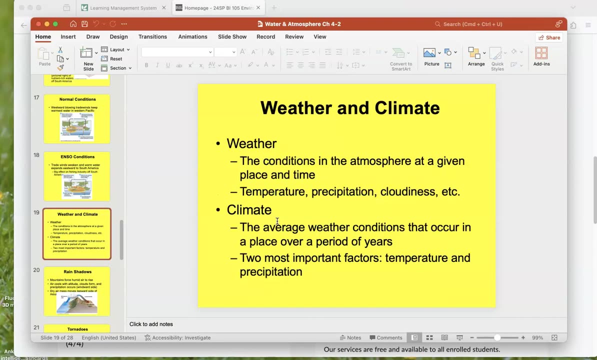 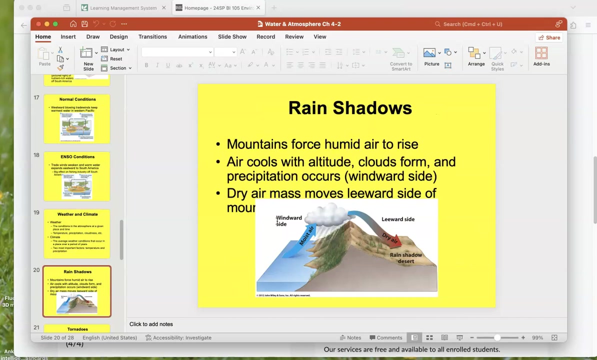 And similarly, we're going to ignore the the ocean currents. Okay, You do want to know the definition or the difference between weather and climate. That's important. Weather is short term, Climate is long term. Oftentimes, like I said, it's not here. I want to say it's like 30 years. is what they look at for 30 years worth of weather to determine a climate? 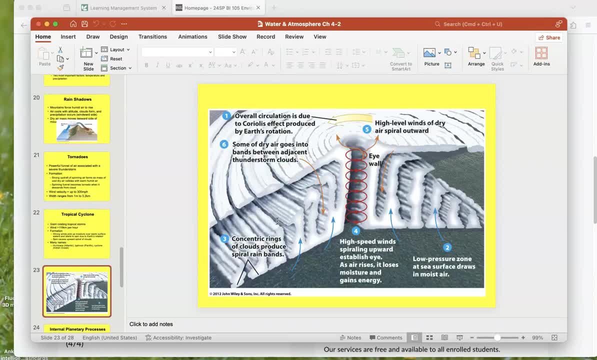 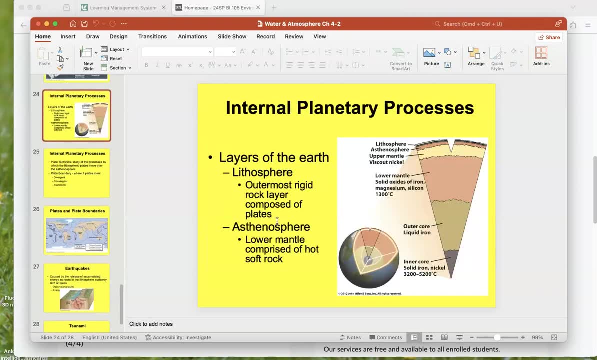 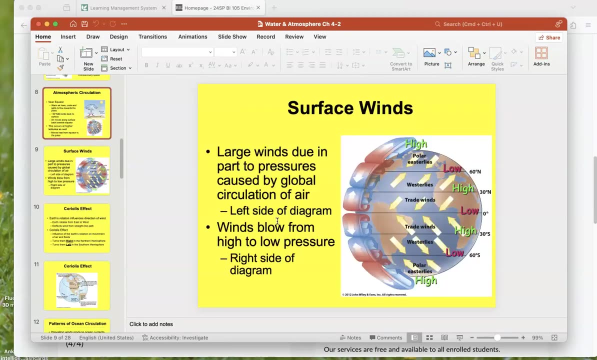 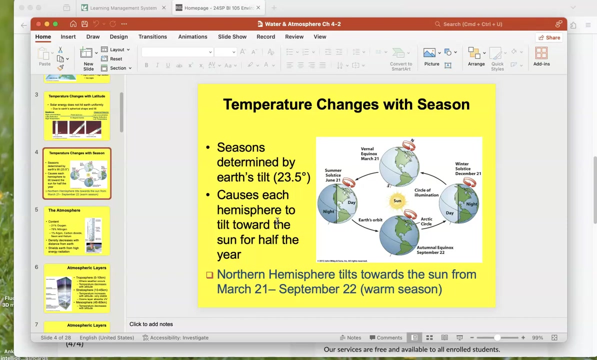 Yeah, And then we just run into randomness. Yeah, So So, difference between weather and climate, Atmosphere and its layers And seasons, and planetary tilt Incoming solar radiation. Okay, That's what we're going to pull out of four. 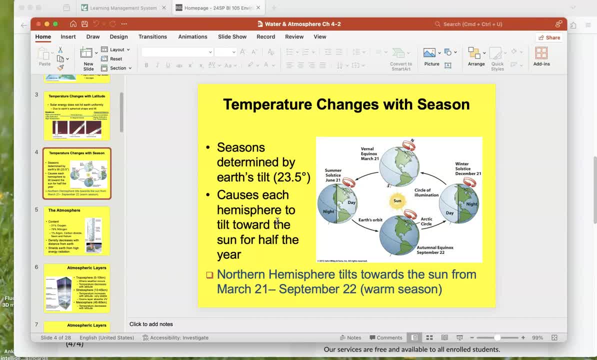 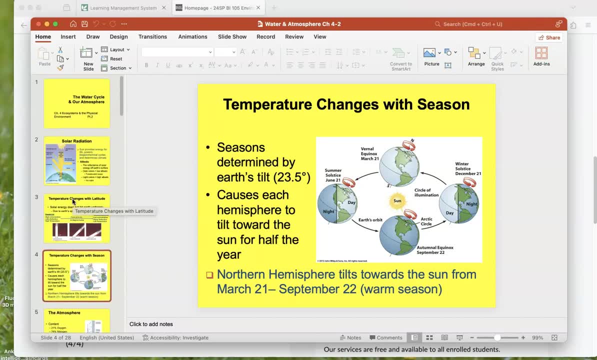 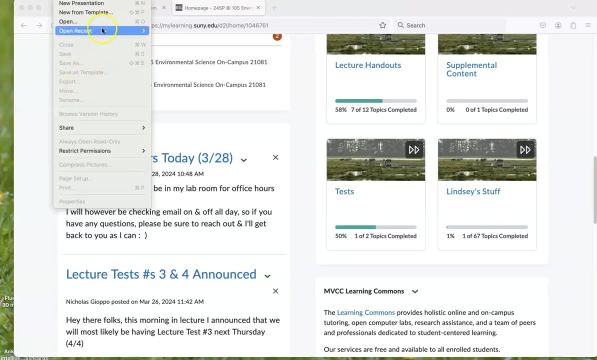 Questions about any of that, Problems with any of that? This PowerPoint is up there, Should you want it. Next thing I want to pull up again. it's almost really just a bit of review. There'll be some new stuff in it, though. 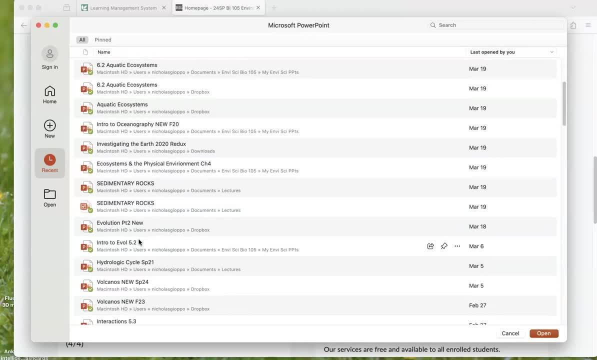 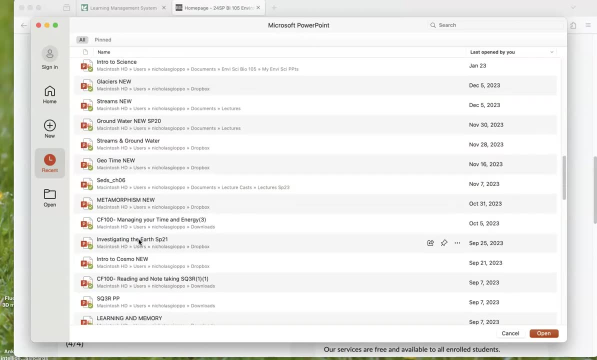 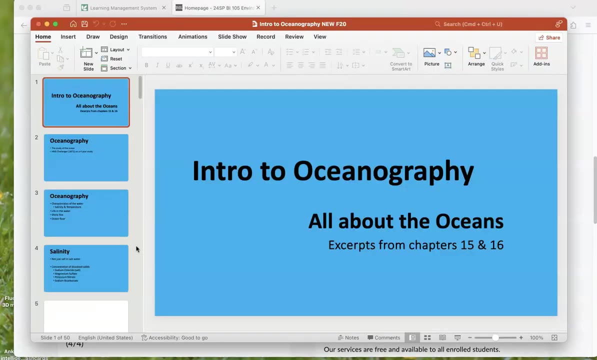 Just I saw a few questions as I was going through the test that I'm worried that we didn't Talk a whole lot about in those aquatic Ecosystems and I hope I'm not Just giving you too much, Too much information. 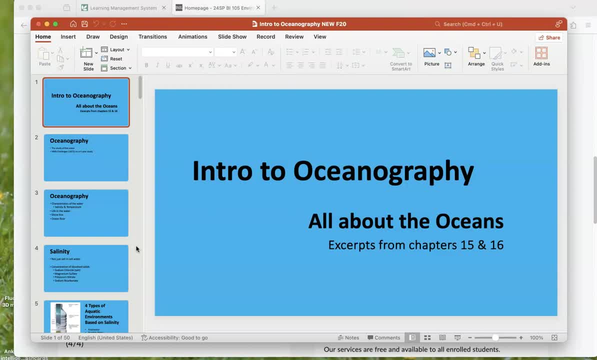 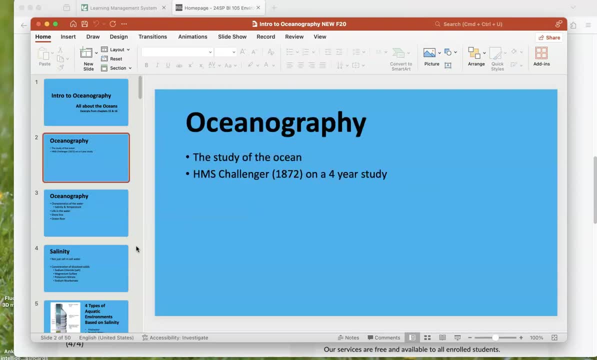 This is actually coming out of my earth science textbook, So when it says chapters 15 and 16, please, you know that's not you guys here in environmental science, but He's not here right now, but he asked a while back. you know, when did we start finding out? 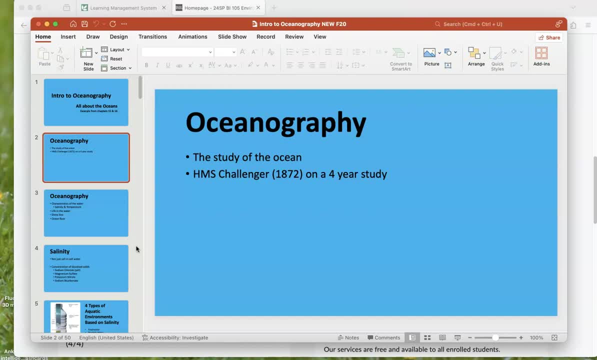 Finding out about all the ocean floor and all this stuff. It was 1872.. The HMS Challenger went out On a four year voyage And I think that was basically the beginning. I do know, again just anecdotal, that during World War Two, with the whole sub wars that were going on, 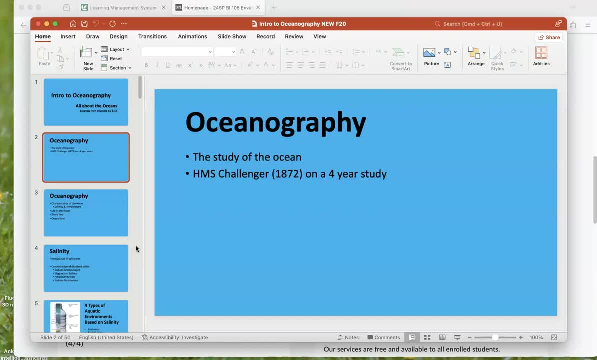 We learned a hell of a lot about the ocean floor that I like, the fact that there's a giant mountain range between North America and Europe called the Mid-Atlantic Ridge- Might have heard about that- And again, earth science classes. It's part of plate tectonics. 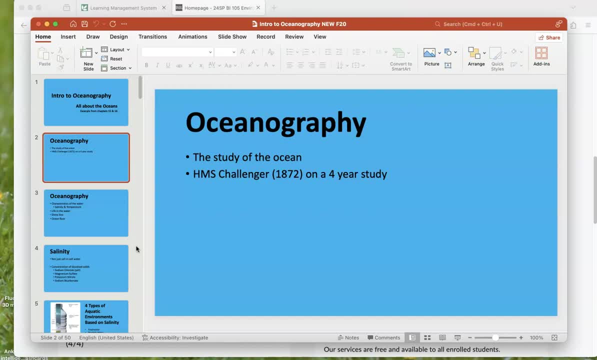 OK, So that stuff came a little later. But some of those islands that are scattered through there- down by Africa, you got the Canary Islands. up by Europe, You've got the Azores- are kind of in the middle there. They're not really by Europe, but those are all bits and pieces of the Mid-Atlantic Ridge sticking out there. 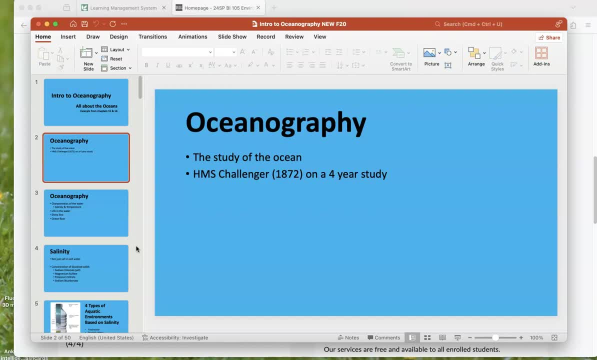 And of course, Iceland is definitely part of that. Yes, sir, Question: My question is not. That's OK, What's up? I think sonar is very similar to that, to echolocation. I don't know if we modeled it off of bats or not. 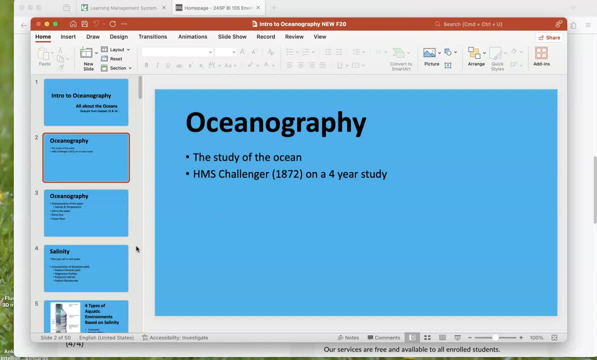 But I know it relies on the same principle: How much time it takes to bounce back to you. You've got to account for an air. Signals travel a lot. Sound travels a lot better in air than it does in water, So they accommodate for that. 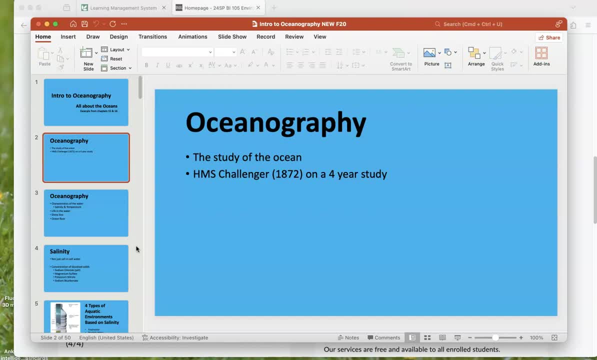 But it's essentially the same idea. Yeah, And I guess you could call it echolocation. They may call it, But I know sonars usually they call it when it's underwater. Yeah, So oceanography as a whole talks about the characteristics of the water which we mentioned. 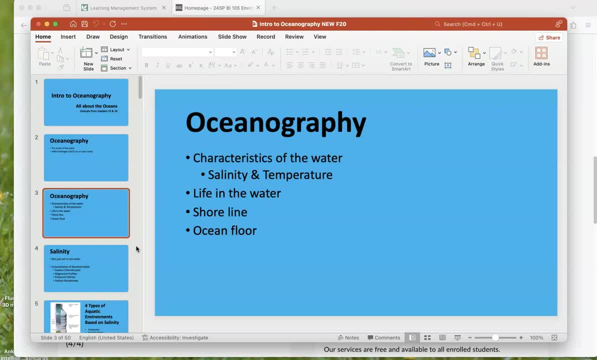 salinity and temperature. OK, Those are the big things when you want to talk about environments. really, How salty is it and how warm is it or isn't it? And that gives us the idea about what kind of life we can have there, plant or animal. 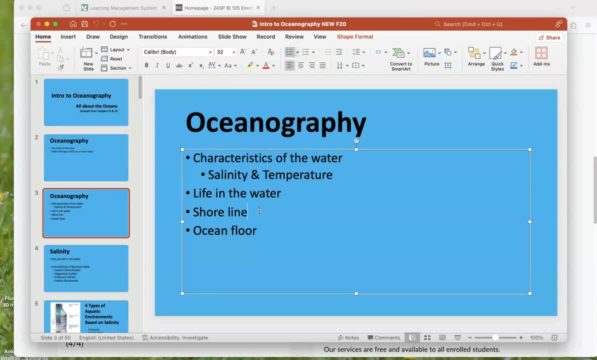 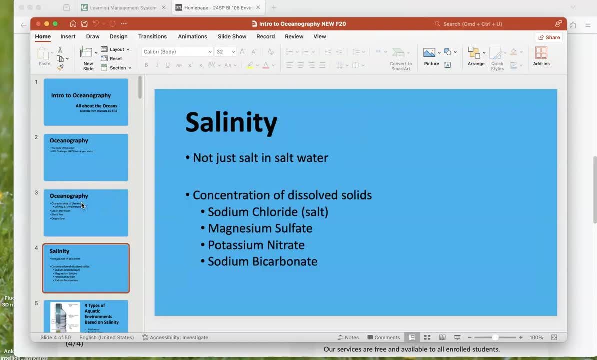 We also have two different general areas. OK, We've got the ocean floor and we've got the shoreline to think about. Oh, since you're back, You asked the other day how long we've been doing studying the ocean. 1872 was the first official HMS challenge. 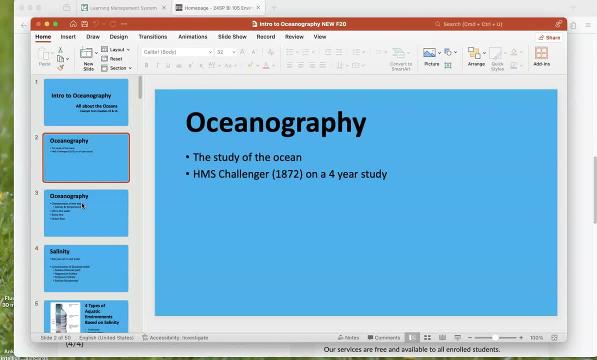 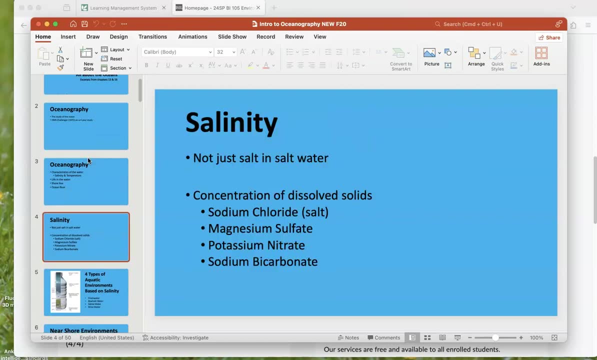 Oh, I know, Yeah, You asked about. yeah. So 1872 was the HMS Challenger. That was the first. There you go, All right. So salinity, we talked all about this. I'm not going to belabor you with more. 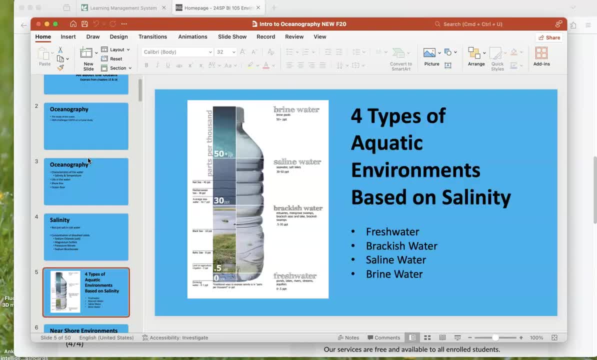 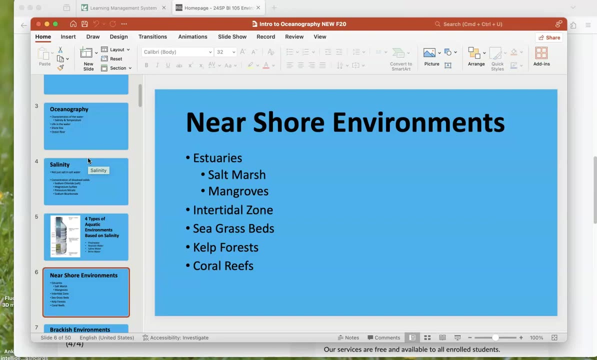 OK, All right, All right, There's that same exact bottle diagram, and why I decided to make it down on horizontal instead of up and down. As you see, it's kind of small, even harder to read. This also again summarizes what we talked about. 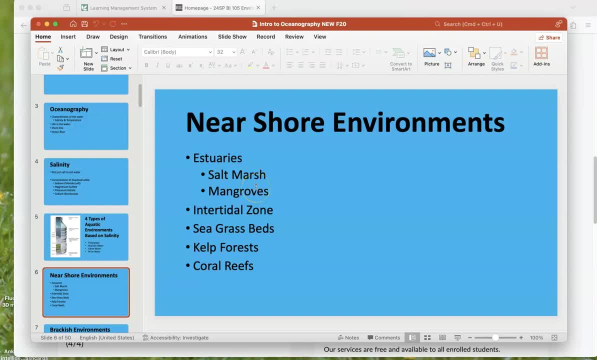 You've got your estuaries, which are broken into two types that we talked about. There's more The intertidal zone. you've got seagrass beds, kelp forests and coral reefs- Kelp is that, the algae on the west coast, those giant forests. 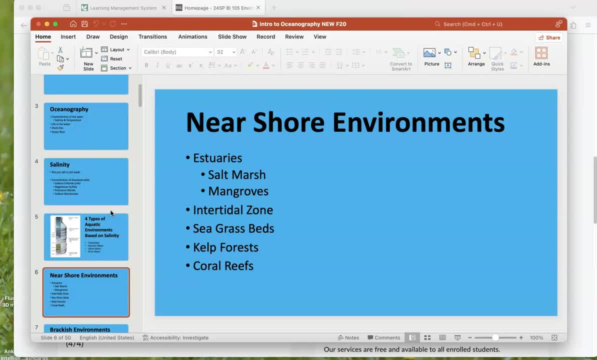 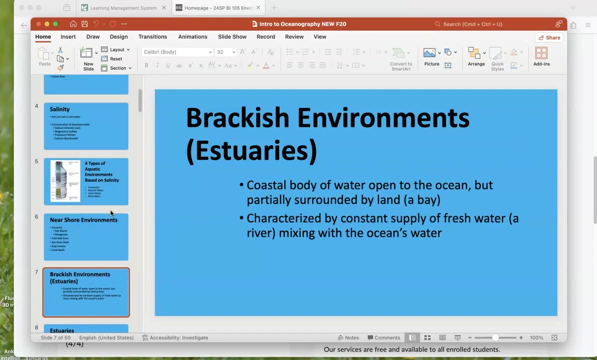 We showed some cool pictures at almost the very end of the 6.2 slideshow, just before we talk about the barrier reefs. This is a review from a slightly different perspective, from an intro to oceanography thing. So these just give you some more definitions. 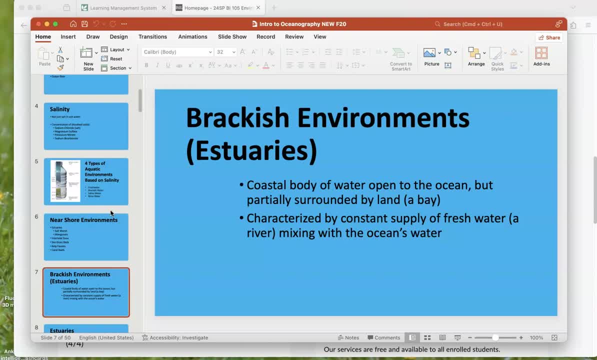 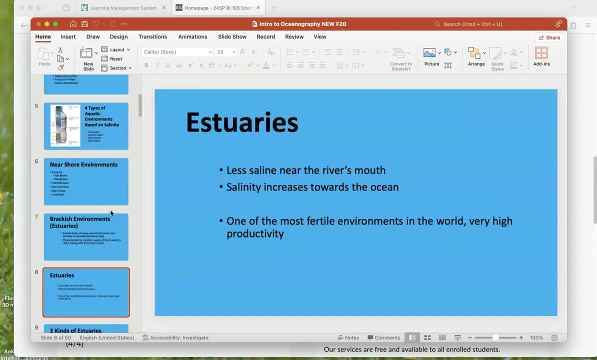 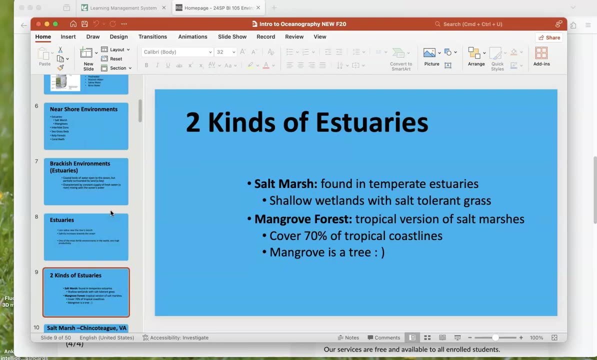 I'm going to put this up. If you guys again find 6.2 lacking, you're going to see a lot of overlap here. The estuaries are the blending of fresh and salty water. We talked about that, The two types that we learned about. 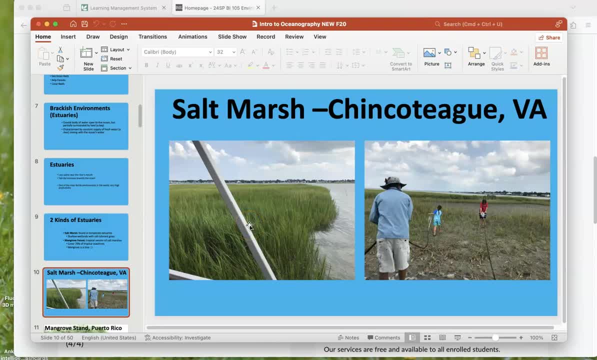 Here is a great example of high tide versus low tide. My wife quite awesomely ponied up for a One of the boat adventure tour things. This guy loved to play Raiders of the Lost Ark music as we were kind of jutting through. 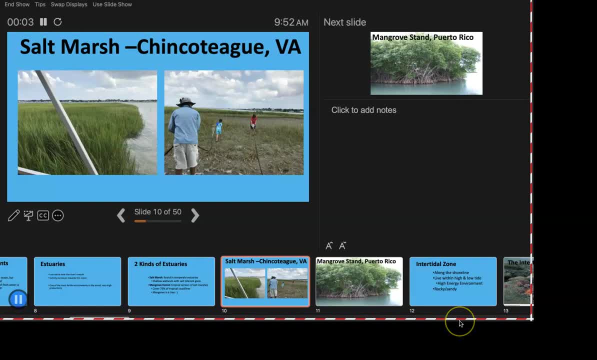 the salt things. He was crazy But it was a good time. It's just some boat rental guide that we did. Those are my children. Like I said, my wife was cooling off the paper and had a little expedition here instead of just going to the beach. 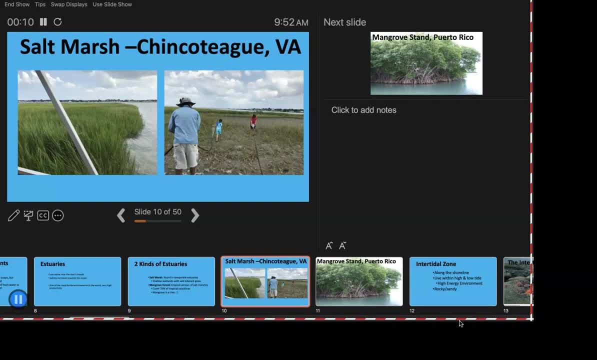 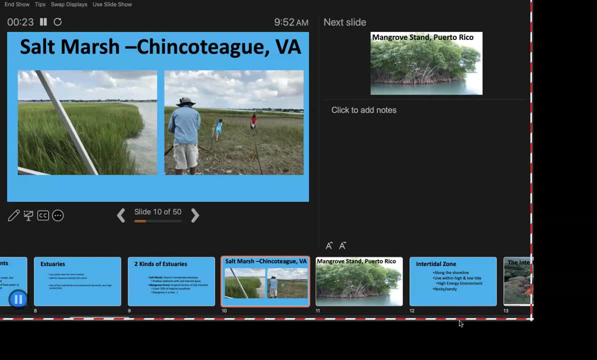 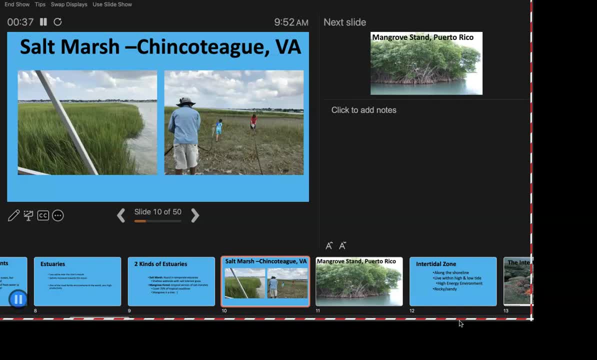 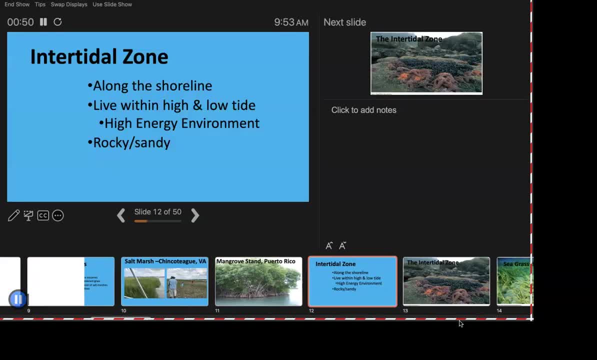 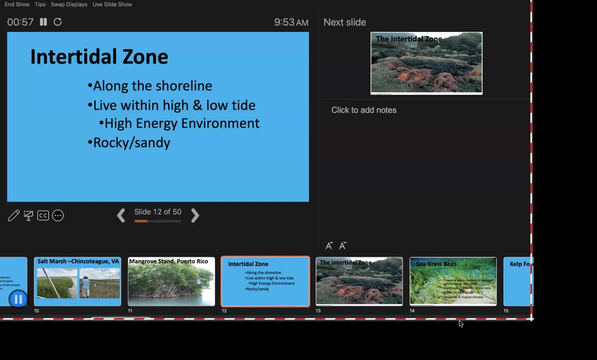 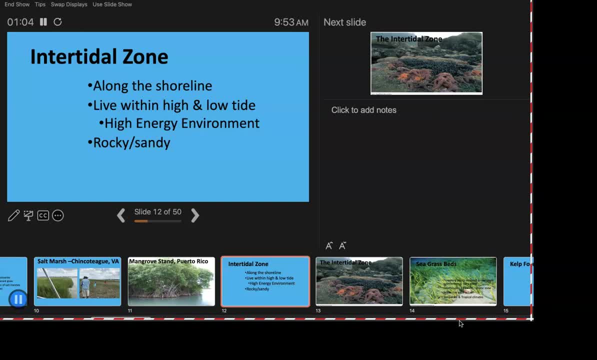 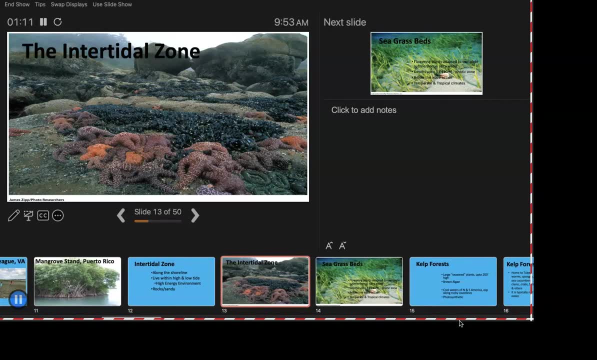 difficult it is to live in that area because of all the it's very active energy. you probably saw this same exact picture. you got our starfishes there and a lot of other, a lot of other critters in the background. when I was in California two summers ago, went to Santa Cruz and we did. finally, I never 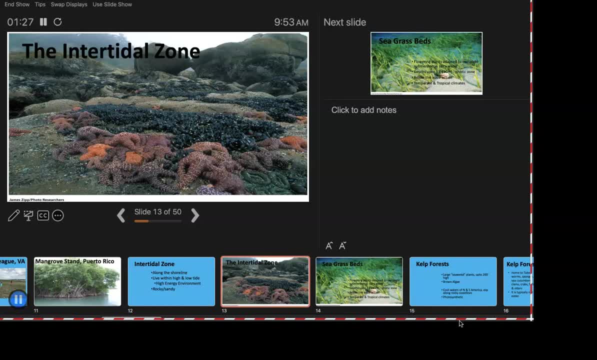 integrated those pictures. I did get to see some life like this. we only saw some, some urchins and anemones, still not seen the starfish in the wild, but just don't, you know, run into that stuff on the East Coast at least where I've been. but I did. 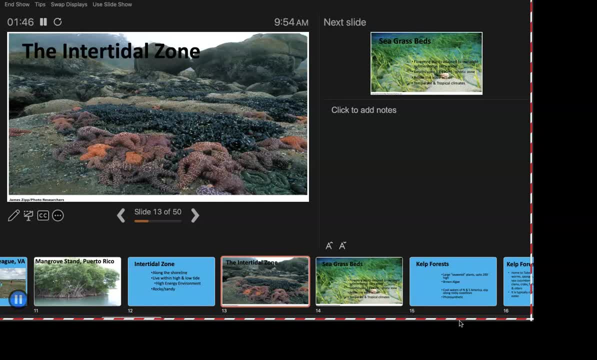 finally get to see a little bit of that kind of life. it is a cool area to explore, slippery as all get out with the, you know, because the rocks are all wet and, you know, slimy, for lack of a better word- but it's. it's definitely worth it if you. 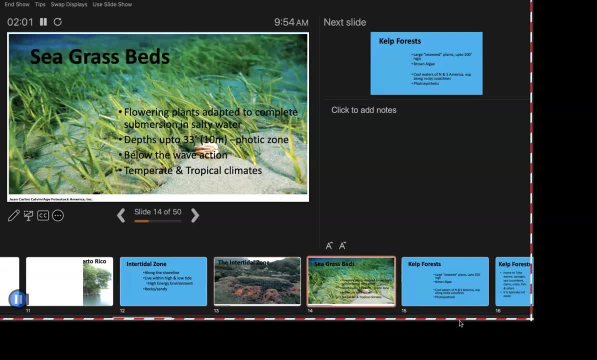 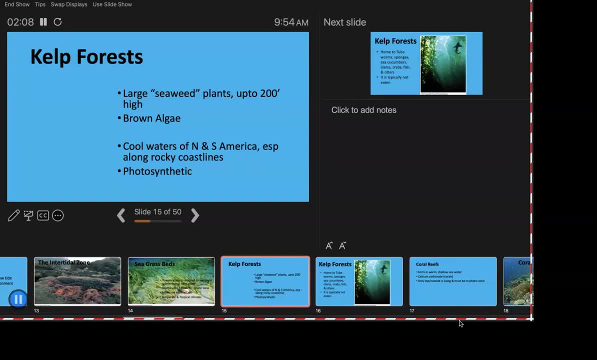 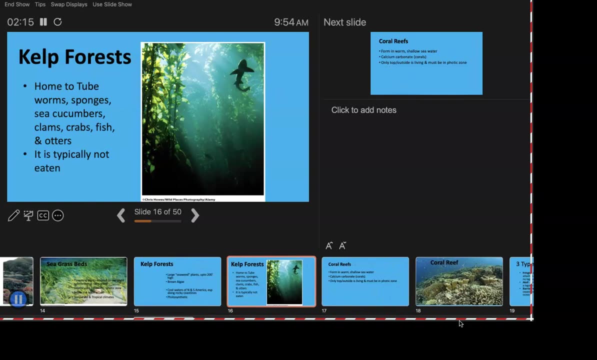 ever go anywhere that you have an opportunity to explore this kind of stuff. seagrass beds- we talked about these guys. you're gonna see your kelp forest again here to answer your question there. this is what we think of as West Coast kind of stuff. it is brown algae and those. these are, you know these. 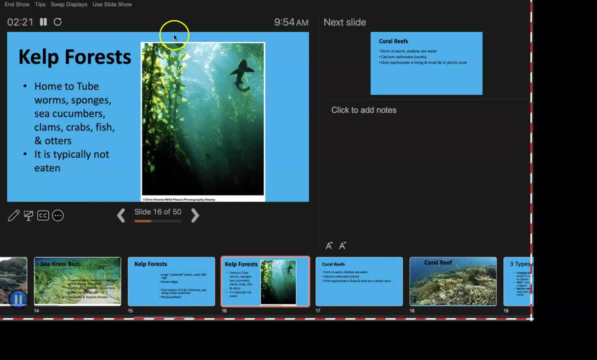 giant tree looking things are the growth structures. we said that they eat live in and around it. they don't typically eat it, but I'm guessing that there's plenty of secondary growth on these leaves that you know you're gonna come along and scrape off with your little suckers and whatnot- like a lot of. 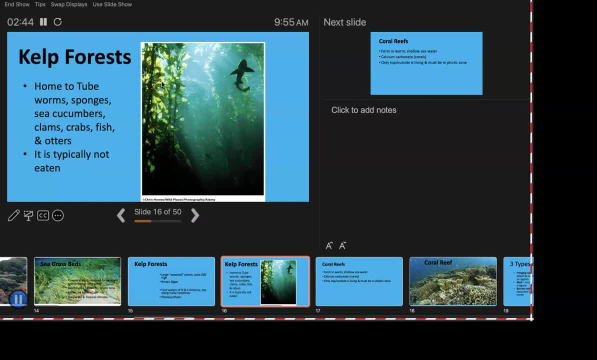 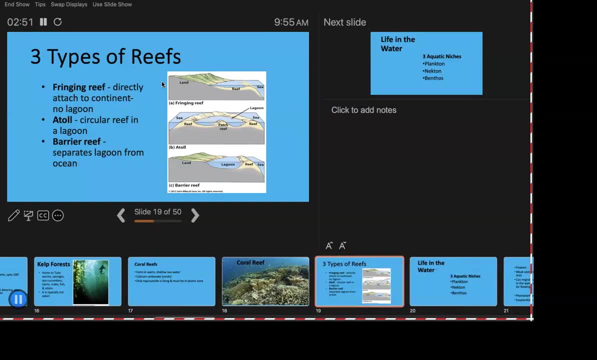 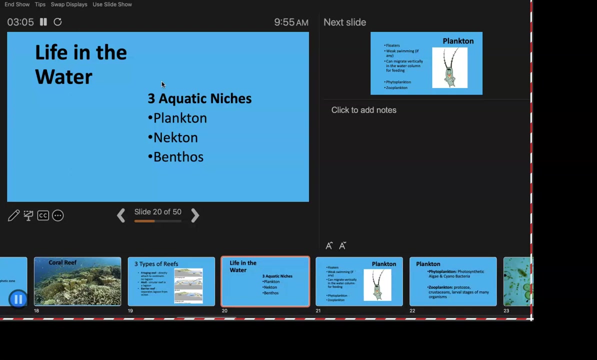 trees, vegetation that provides home for secondary growth. we talked about the coral reefs. there's the three types of reason. this is, you know, really just a rewrite of that PowerPoint. I just think it's slightly better. all right, so, and this is the main reason, this stuff is on the test. the plankton, the neckton and the. 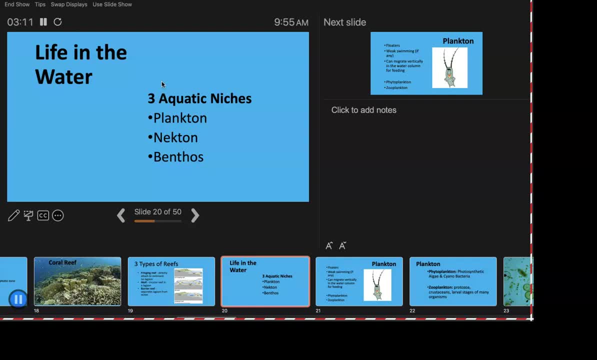 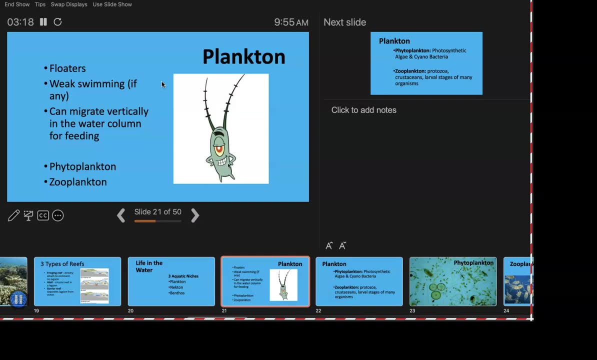 benthos, and I was just worried that it was buried in the content from the other one. all right, talks about your two types of plankton. your fight phytoplankton and your zo plankton. you yep. so the plankton are weak swimmers. if anything, they're primarily floaters. 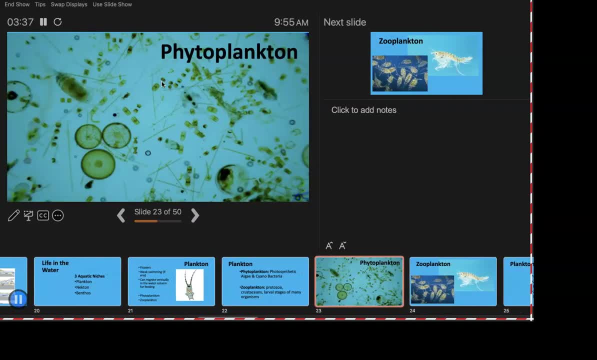 okay, there's some pictures. we didn't have those before, so maybe you see now where they got a little inspiration for the mr plankton there. what you can't start the sentence. I've got a good question and then go to fun club, but go ahead. 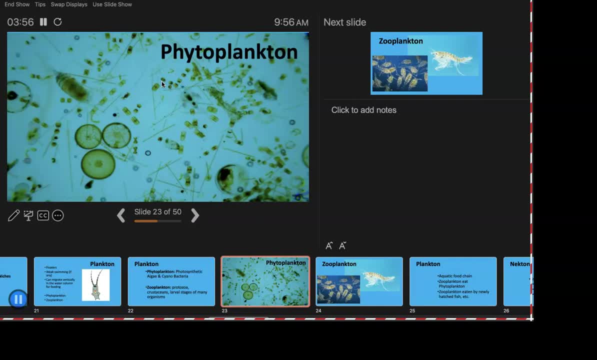 I think the better question is: how is his daughter a whale? anywho, and again, the star is starfish is supposed to be smarter than the sponge. that's all I will say. he's not evil, yeah, but Patrick is coming to the rock, got smart. I remembered, and in the beginning he wasn't. he wasn't active. 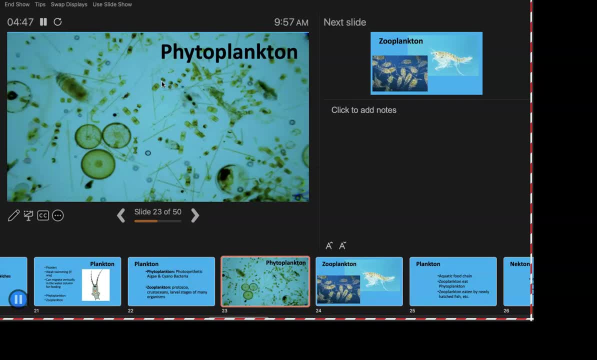 he didn't quite act as an earlier épices. I've heard them all a million times cuz they were in the backseat while I was driving, but I bought. this time I've stopped to see them there. after talking to them, you adapt to it on TV as well. SpongeBob kind of replaced. 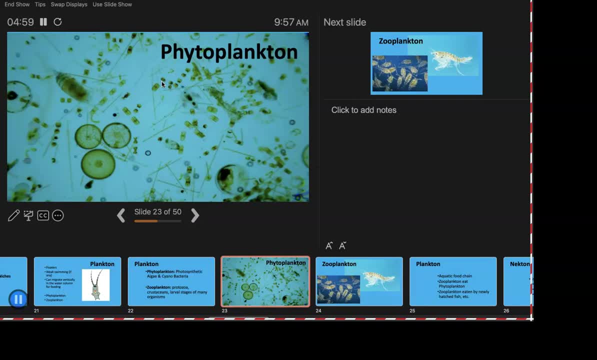 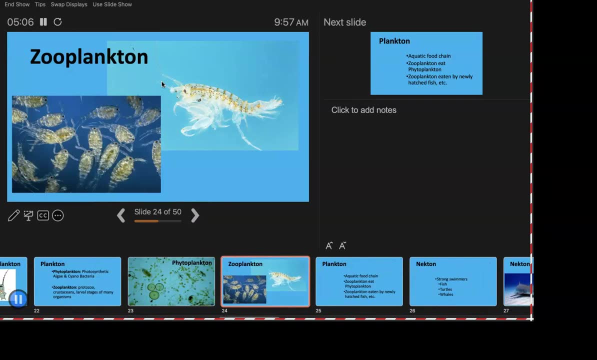 Pauly Shore movies. for me It's mindless entertainment. Here's some zooplankton, Some examples. That was Fido on the previous screen. Teeny, tiny little guys You hardly ever get the chance to see, but you know they're moving by you in the water. 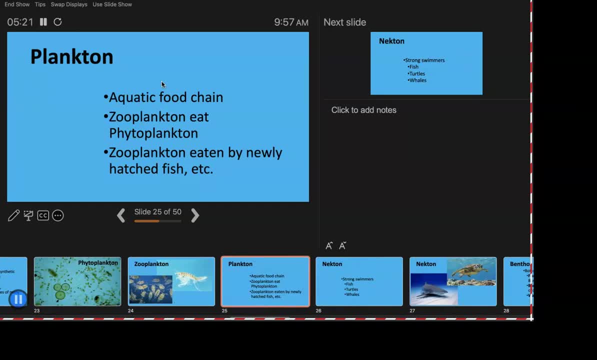 And again, plankton is definitely part of the food chain in the aquatic systems. The zoo eat the Fido and the zoo are eaten by the slightly larger critters. The Fido is the base of the food chain. Also there is some free-floating algae and stuff like that. 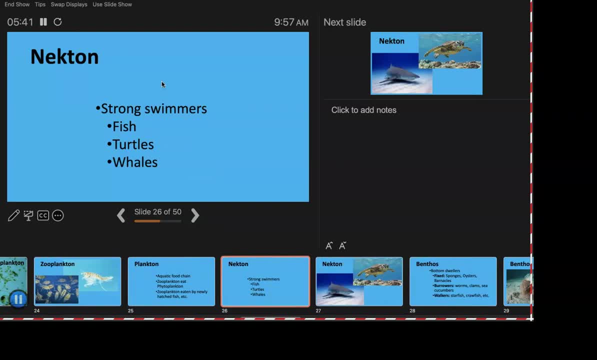 So, moving on to Nekton, Nekton are your stronger swimmers. I just randomly picked fish, turtles and whales. You could have said marine mammals, Reptiles and fishes. Fish are the same level of classification as reptiles and mammals. 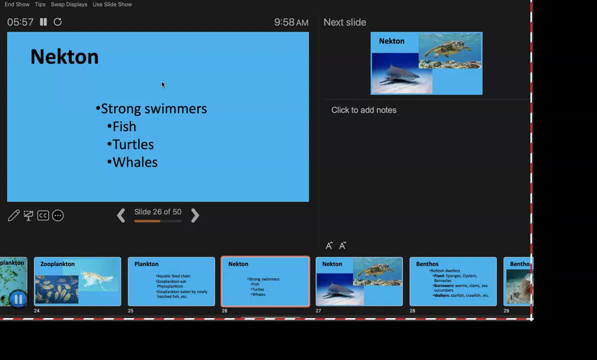 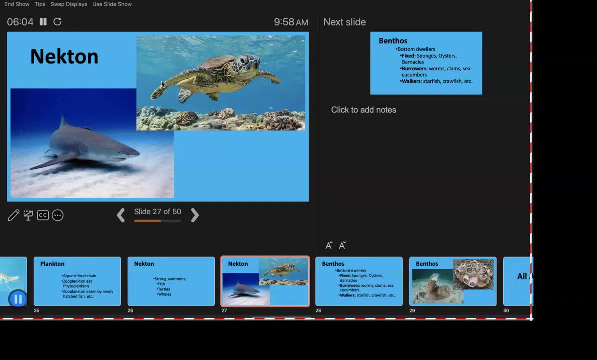 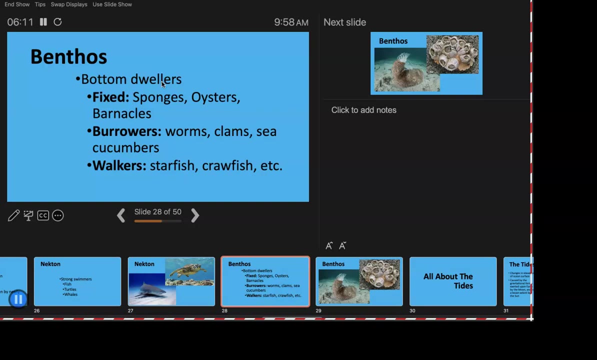 They're both classes. If you didn't know what I was talking about, there's some pictures. Benthos, bottom dwellers. We told you there were a couple different ways to live on the bottom of the ocean. You could be fixed attached Sponges, oysters, barnacles. 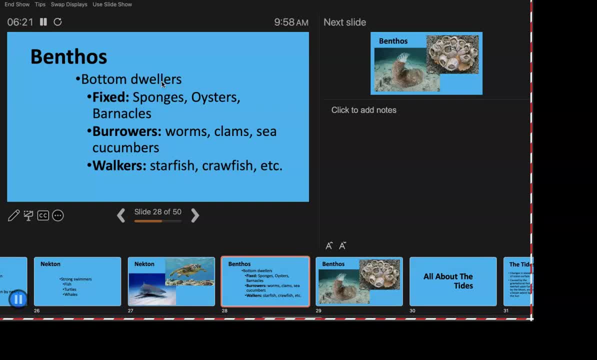 You could be a burrower- Worms, clams and sea cucumbers- Or you could be a walker or a crawler, whatever you want to call it- Starfish, crayfish, etc. So we've got some barnacles here in the upper right. 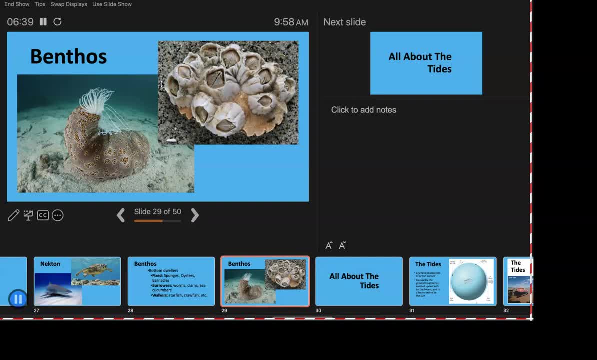 Barnacles are very cool. The thing that looks like a kind of really weird pupil. there is an opening or closing They can, so they live in that round shell, kind of like a tulip-looking thing, And that opens up in this. 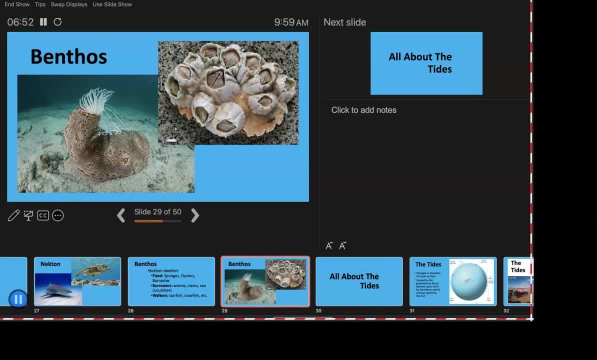 And this cool little waggling creature comes out and filters. these Barnacles are a pain in the butt. of course You see them on a lot of posts If you go near the shore, like on dock posts and so on and so forth. 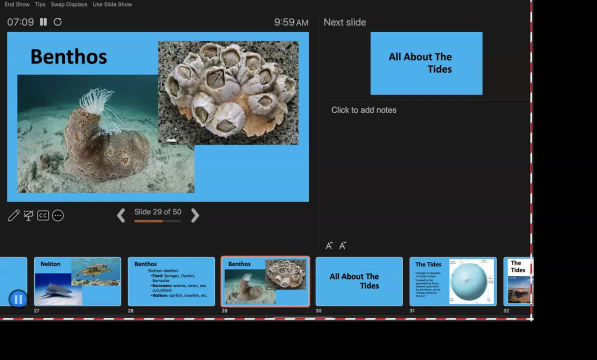 Again, it gives you an idea of the tide level And apparently they're a constant pain for boats. They have to scrape them off, and so on and so forth. Yes, sir, your question. They are unique. They are unique, And what's really funky is that thing on the left. 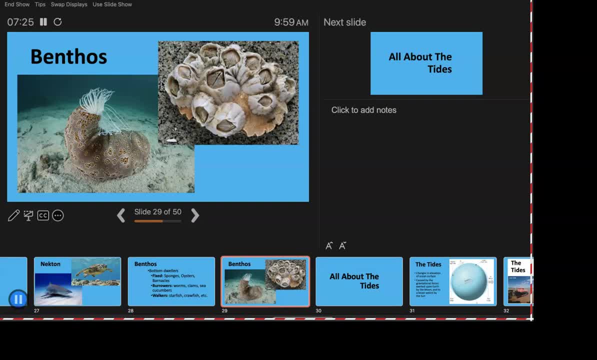 Anybody have any idea what that thing on the left is. That also is a structure. That's pretty. Huh. I heard somebody in the back- The barnacle's upper right And this guy down here on the lower left. You got a hand. 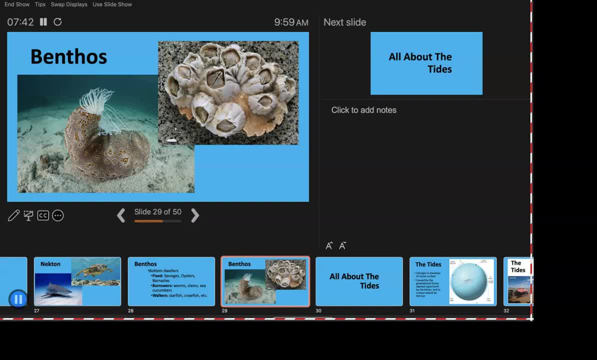 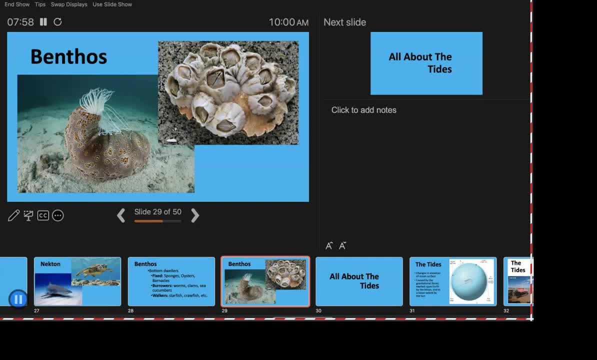 No, it didn't actually do that. So again, anyone for the picture on the left Sea cucumber? Yes, thank you, And it's a really funky pattern. Oh, barnacles, Yes, Yes, Is they young, Like up close? 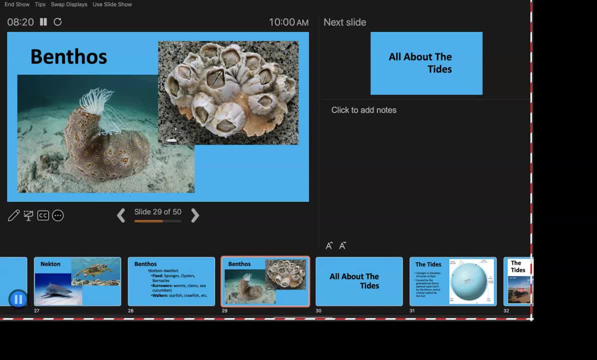 They don't usually get that. Yeah, that's a nice. it's, you know, taken for educational purposes, right, But I don't want to see you guys do it this time, All right? Well, let's quit talking about it and I will change slides then. 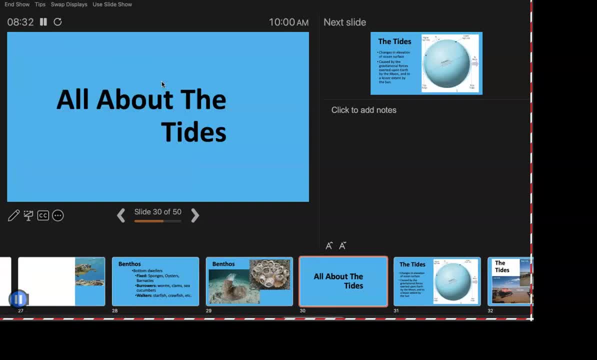 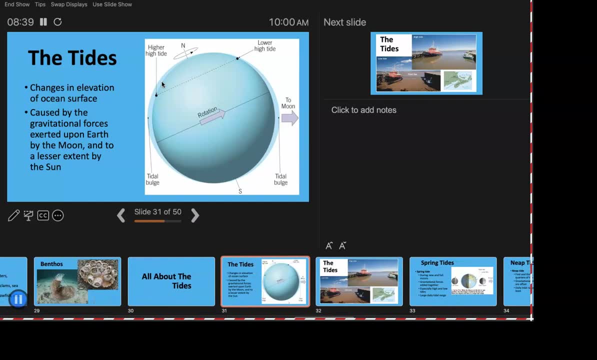 Yeah, But I think the sea cucumber's really kind of cool looking. All right, All right, This is new and this is kind of worth knowing. So I will put a couple questions from here on the test. The tides, all right. 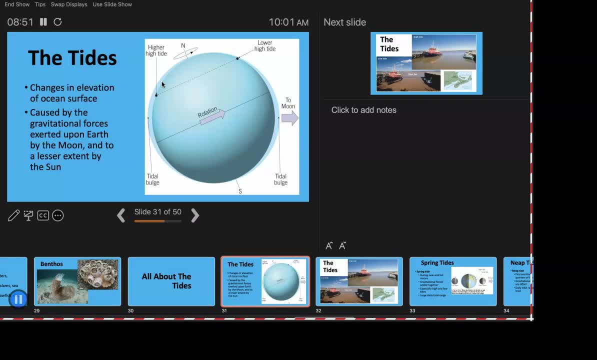 What causes the tides? Before we go any further, The move and the gravity. because of the move right, All right. So the moon's pull on the Earth will move the ocean water, It's that powerful. As it moves around, it changes how much it pulls. 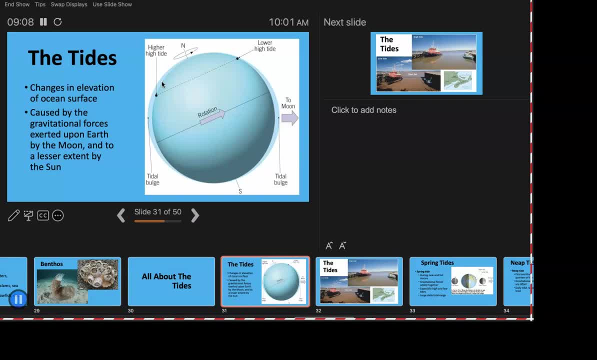 Sometimes it's farther away, Sometimes it's closer right, And sometimes it's on a different side of the Earth, So that's why they change as well. The ocean: Yeah, Can you talk a little bit more about that? Because it's so far away from the other side of the water. 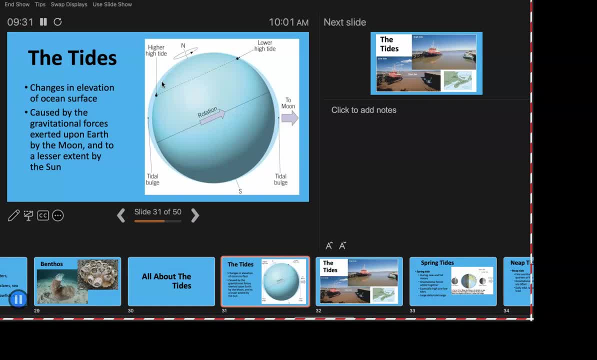 Stop tiding, Yes, And the moon is slowly but surely moving farther away. It used to be a lot closer. No, She means farther out in orbit, I think. I assume. Yeah, No The less the tides move. 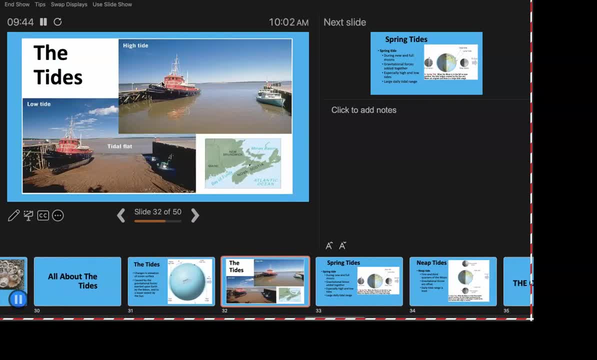 The less sea level tides move. Yeah, Yeah, Yeah, Yeah, Yeah, Yeah Yeah. That's one of those things. For example: all right, high tide top picture, low tide bottom picture. that boat isn't. 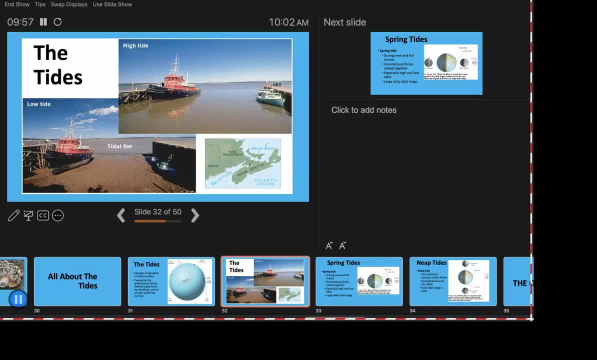 going anywhere. It's not usually that extreme Again picture chosen for educational purposes only, But it gives you an idea. I wanted to give you an idea Again. if you've been lucky enough to get to the beach, you're familiar with this usually. 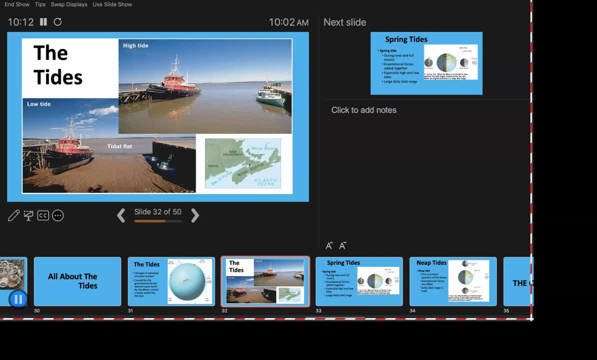 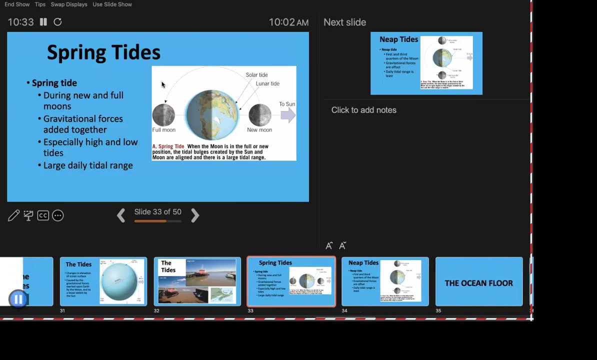 with lawn, chair and or towel placement. Okay, Nova Scotia, So Nova Scotia, Nova Scotia, Nova Scotia. That might entirely be what it is. I never thought of it that way And I'm not All right. so we got spring tides. 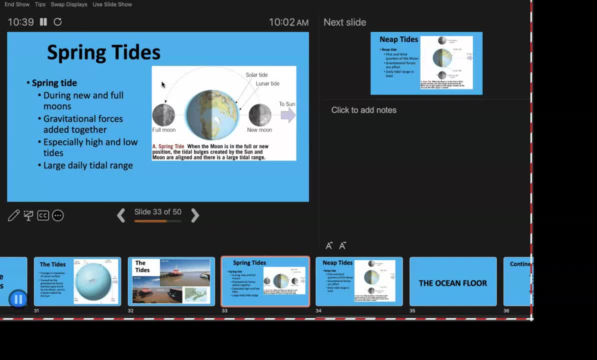 Spring tides. Spring tide you get during a new moon and a full moon. We all know what a full moon is. What would you consider the new moon? Huh, What's it? look like Nothing exactly. So it's all black. 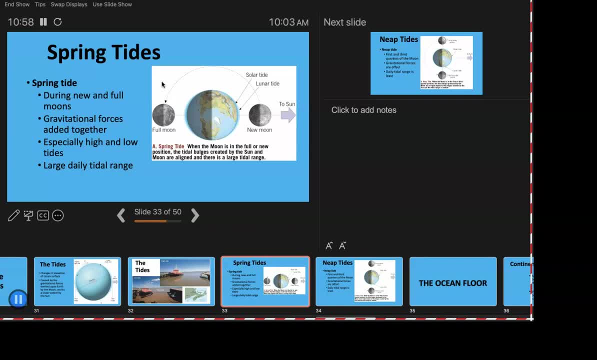 You don't see a moon, All right, it's there still, But new moon is all gone. So you only get those twice in the lunar cycle there, Well, I guess at the beginning and the end. So you get, And this is kind of 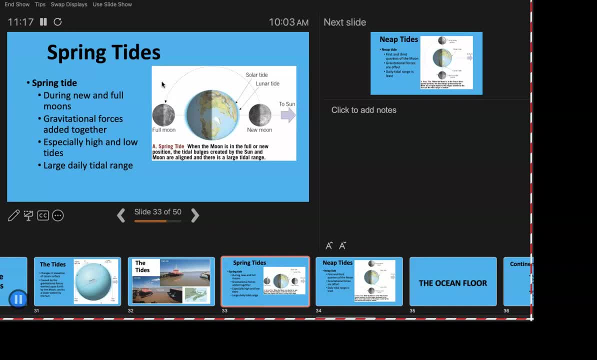 I don't want to say kind of confusing. I don't want to set expectations, But because you're combining your, Excuse me, I think I'm done choking Because you're at that special point where you're seeing a 100% of it. 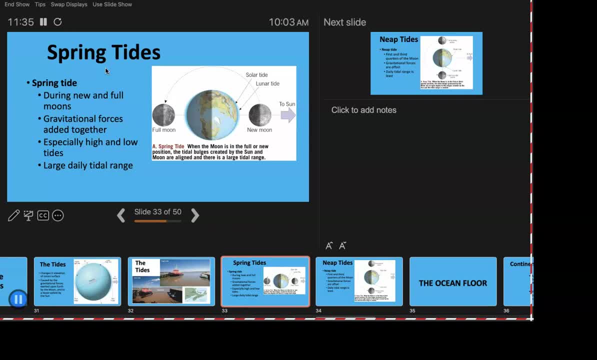 whether it's blocked out or not. that means it's lined up in such a very specific way. Okay, And what that does is it gives you exceptionally high and exceptionally low tides Tides. So during During a spring tide, you'll see these larger ranges than usual. 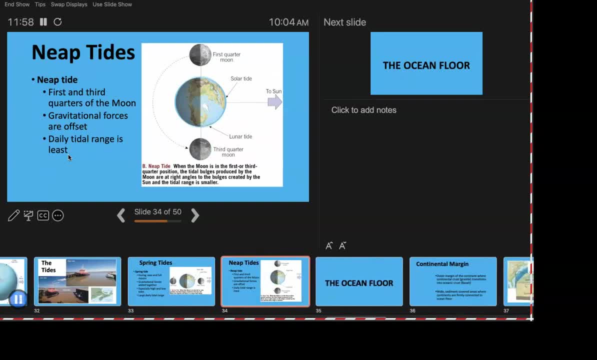 During a neap tide, all right, we see those during the quarter moon And again, the placement is such I don't want to get into the physics of it. It's actually kind of hard for me to explain the physics of it. 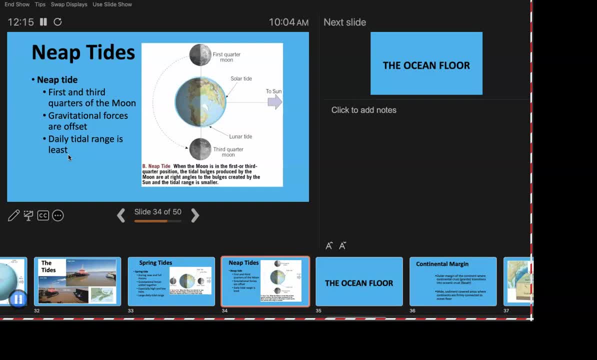 why the gravitational forces are doubled in one situation and not in the other. I apologize, But it's a bit beyond me. These are the least tides, So neap, I don't know. think of it as a noise that a small, tiny little animal makes. 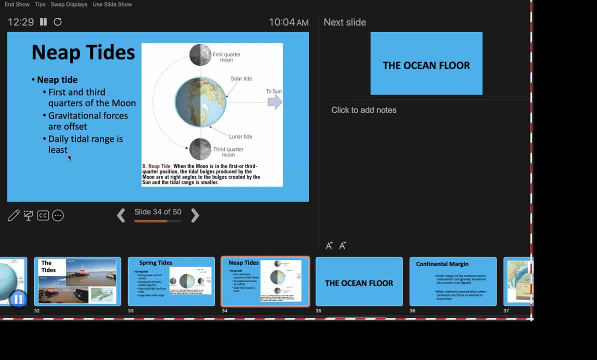 So, on a neap tide, you're going to have the smallest changes, But a spring tide, you're going to have the biggest changes. All right, I won't ask you about the moon phases. I promise you that, So you can actually 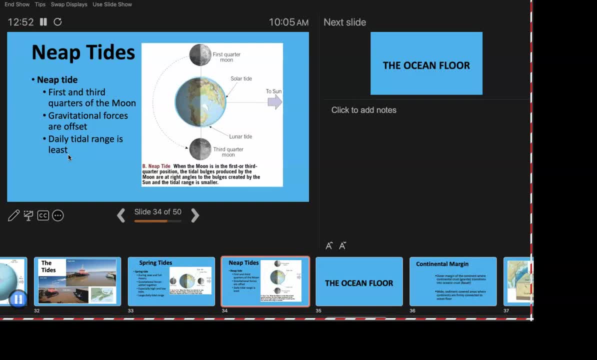 And we can predict these. We know how the moon moves. All right, We know how it affects us. You can look at tide tables And you can, you know, plan accordingly, because those have effects from fishing to surfing, to, again, all kinds of things. 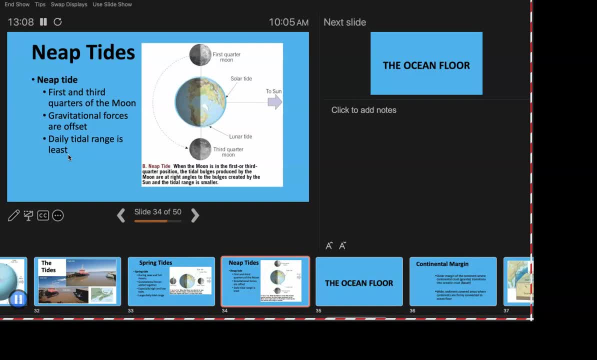 even in the right season to mating and whatnot. So fairly important. And yes, the sun, as it says, is a very important thing. And yes, the sun as it says is a very important thing. And yes, the sun, as it says, is a very important thing. 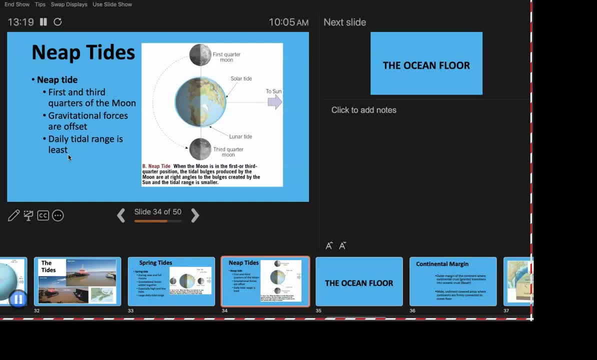 It does have a little bit of effect, but nothing as consequential as the moon. even though the moon is a fraction of the size, It's way closer Again. you're talking about 250,000 miles for the moon on the average to you know, 93 million for the sun. 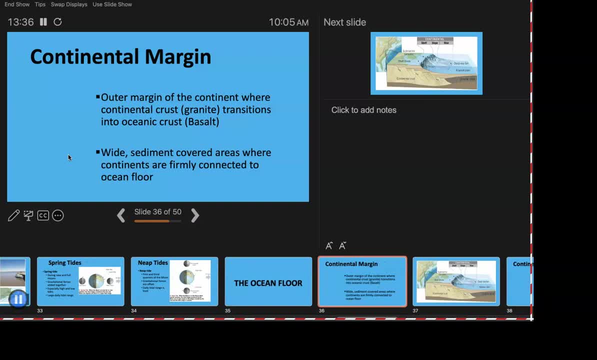 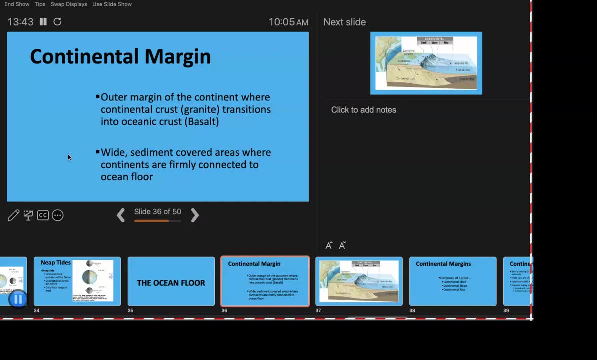 All right, Again, this stuff is in 6-2.. I just think this is a bit clearer explanation. So we had the number of continental slope, continental rise, continental shelf, those terms. there are questions about them And I just want to make sure that you have an opportunity to hear that stuff again. 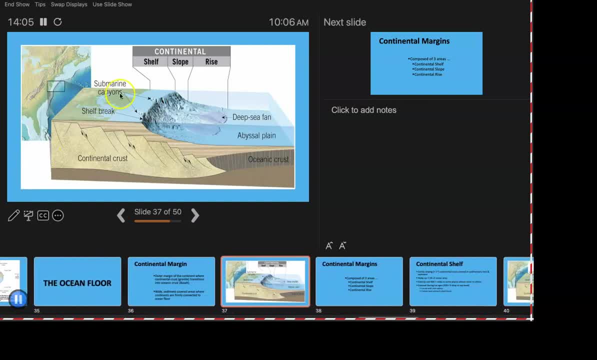 So, looking at a diagram here, this is the shoreline. obviously This is deep sea. So the continental rise: you're approaching the shore, The slope is the really steep part And then, once you get to the shoreline, you're going to see the slope. 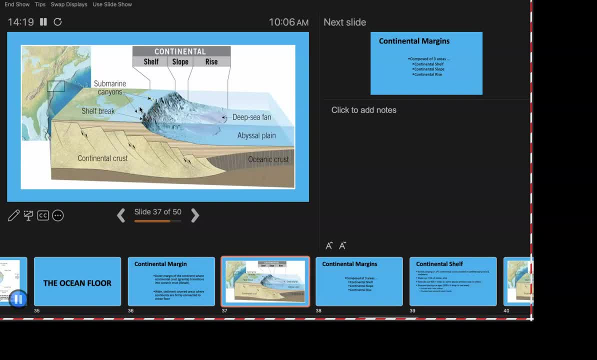 And then, once you get to the shoreline, you're going to see the slope. And then, once you get to the shoreline, you're going to see the slope. And then, once you get up that slope, you know, I think they should have called it continental cliff. personally, but whatever, 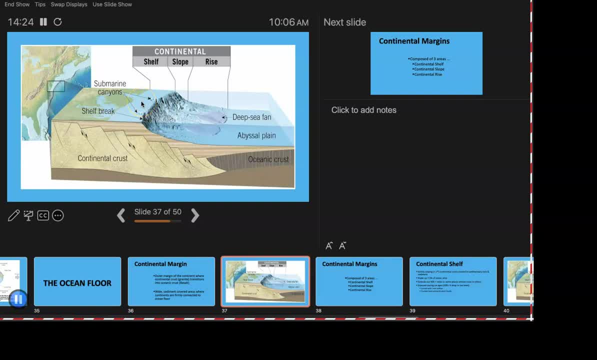 Once we get up here, the continental shelf, all right, is there? Just in case it doesn't come up in another slide, I think it does. The continental shelf is continent, all right. The rise. The rise is ocean floor, if I'm not mistaken. 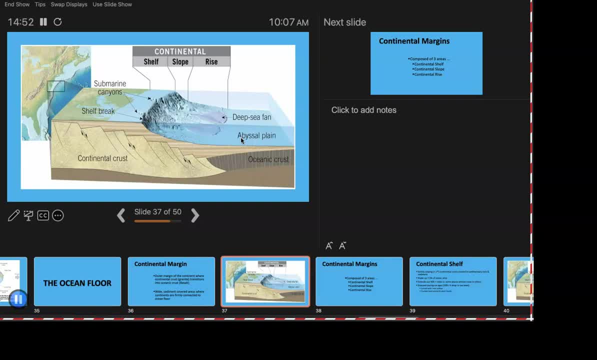 We'll hopefully verify that in a moment- And where the two combine. you guys, we didn't get to that in here, But the continents are made of a rock called granite And the oceans are made of a rock called basalt. You don't see either of those because of all the sediment on top of everything. all right, 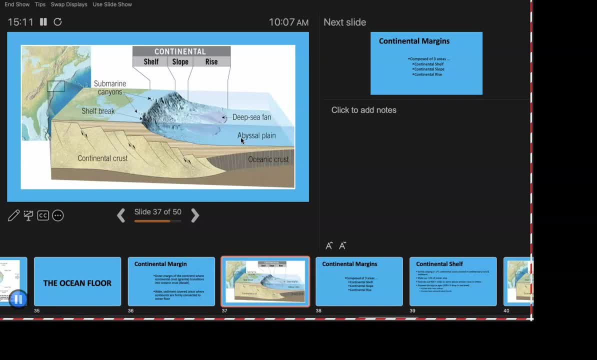 which is what this diagram is trying to show you here. But yeah, so, and here's the split Way down here, and this stuff that looks like wood grain, that's your sedimentary rock on top of everything, which is neither continental nor oceanic. 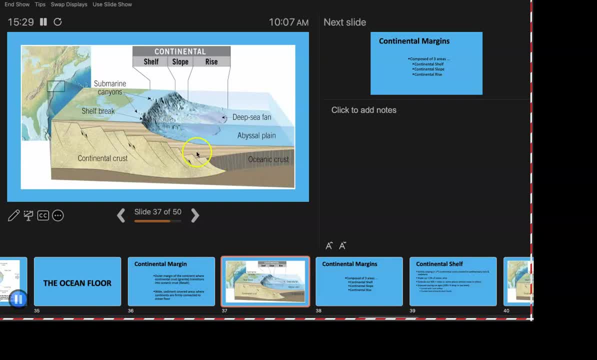 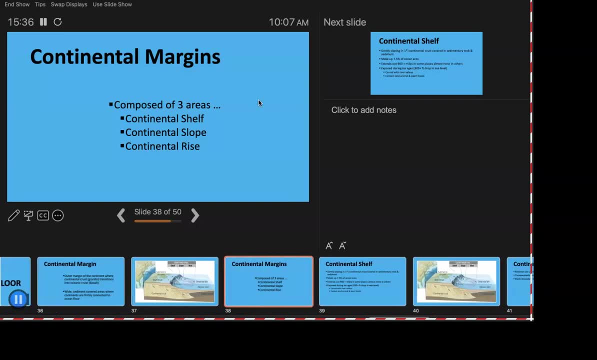 So we get that split here, where the rise is the end of the ocean but the shelf is full on continent. So let's see here. So your continental margins, composed of three areas: the shelf, the slope, the rise. Don't worry about angles. 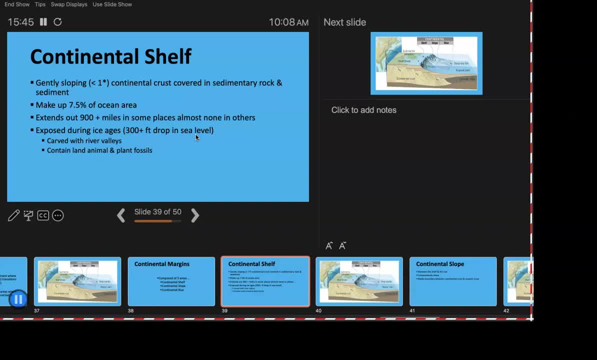 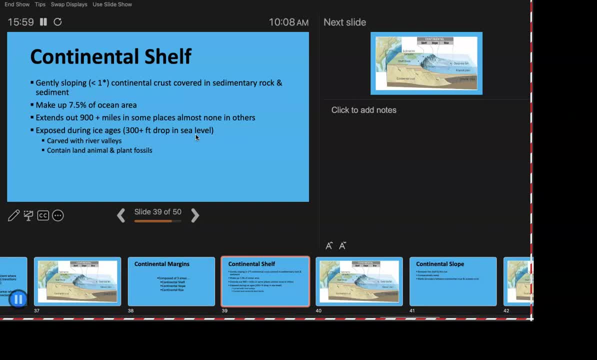 And again, if you're wondering why that is water cycle, We only have so much water. You're going to cover the continent with giant glaciers. That water's got to come from somewhere. It came from the sea, So sea level then went down. 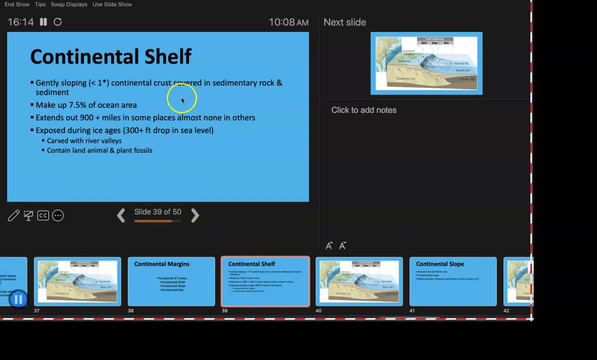 And what is now the coast? you know, you would have been, as it says here, oftentimes the home of the town, but it doesn't. We're talking about the water level increases, the European Ocean? Well, it doesn't. 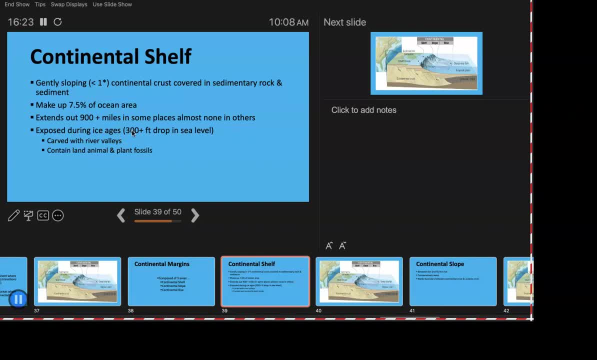 A 300 foot drop in sea level, though, so you can extrapolate that outwards to many, many, many miles. Oh, and also we find land animal and land plant fossils in some of those rocks. if we could, you know they're hard to get to, but when they do find them, 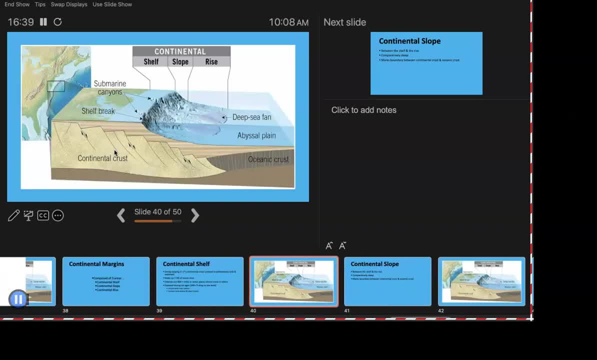 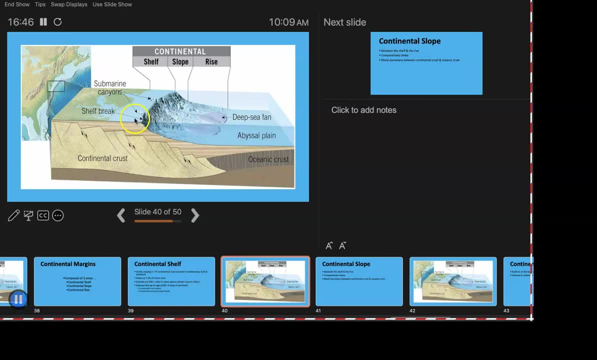 So that's how we know it was land. So again, that is up here And it's easy to imagine. So under the soil, Imagine sea level going out significantly further out to maybe here That's a big difference. 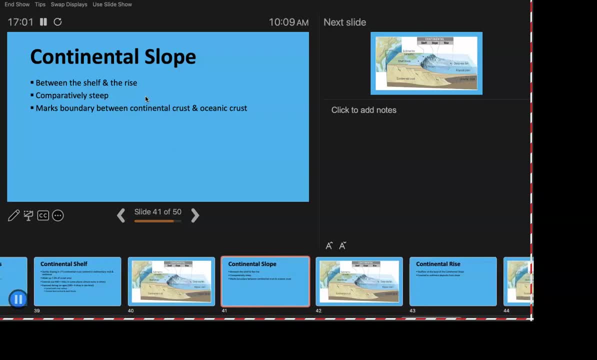 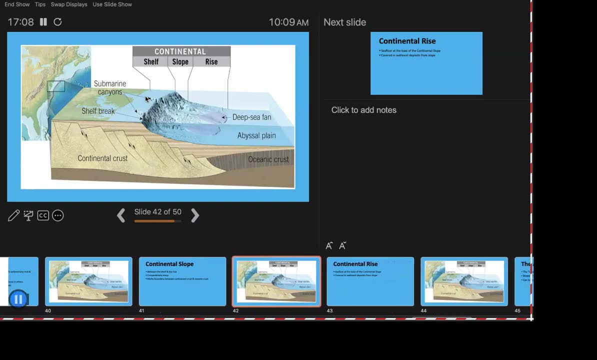 Continental slope. I joked about it being called the continental cliff. That marks the boundary between the continental crust and the oceanic crust. Nothing else really significant there. If you were walking, it would certainly be, like I said, a very bad fall down that cliff, face there. 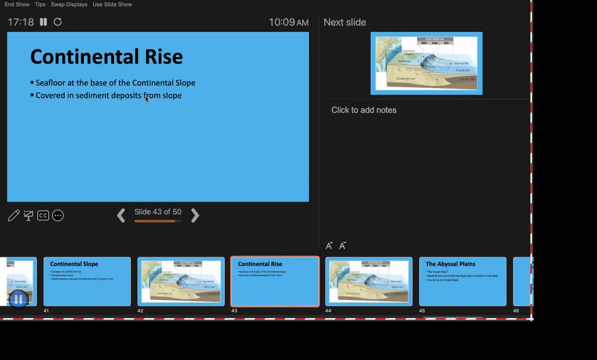 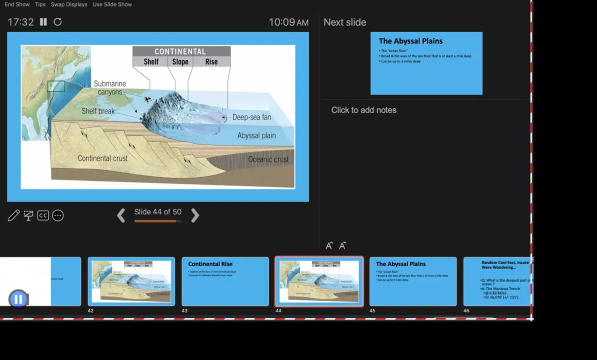 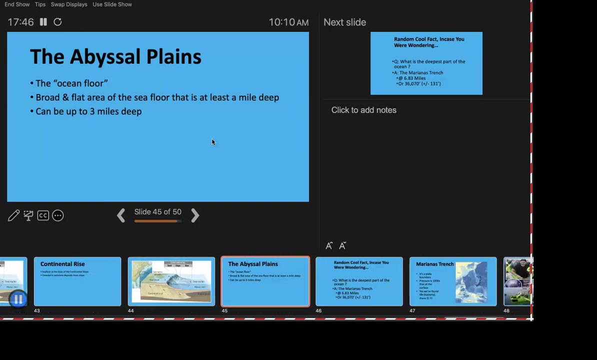 And then the continental rise. This is the ocean floor. It's still a transition, but it is composed of ocean rock And again, all this is covered by sediment that has washed down here over the years. The abyssal plain- The abyssal plains is arguably, not arguably- just a straight out. the ocean floor. 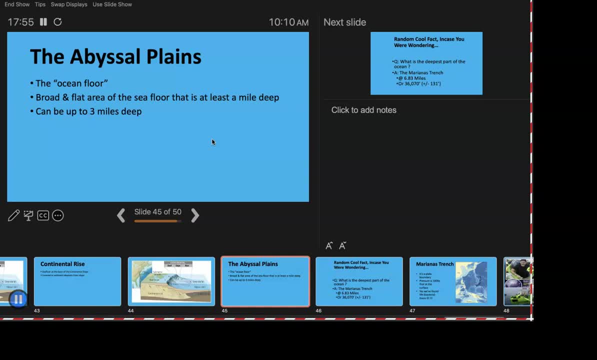 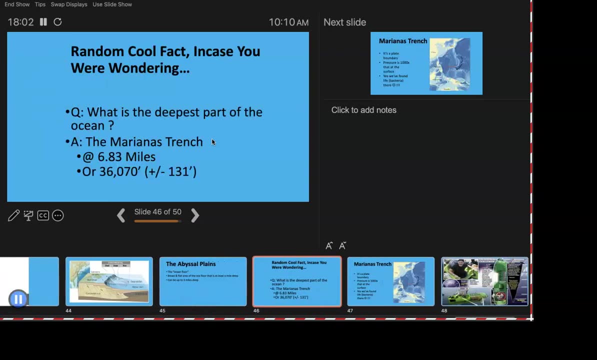 Broad flat area At least a mile deep out there. Of course, it can go as deep as it wants to. We talked about the Marinas Trench the other day. How deep can it go? Well, apparently, almost seven miles deep. 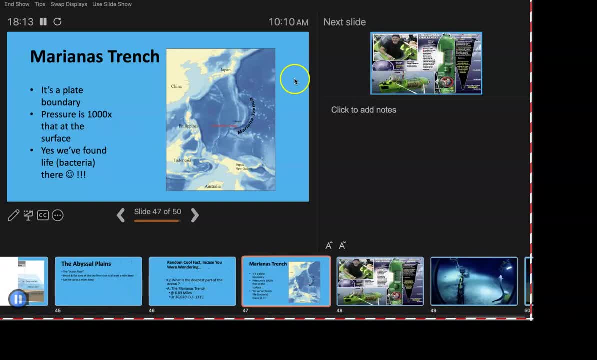 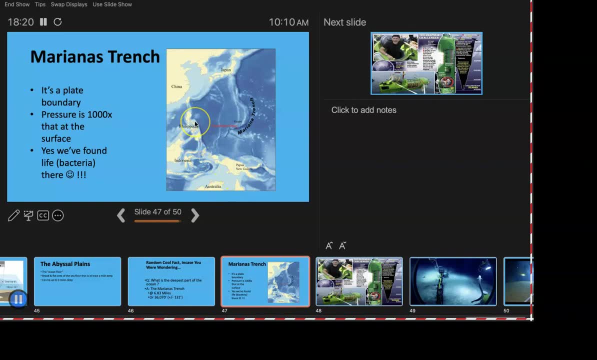 36,000 feet That's out in the Pacific Ocean. We've got Australia here, Papua New Guinea, the Philippines. if any of that is any help to you, Here's Japan up here. So over what we loosely call, going back to how generic things were in the 80s, 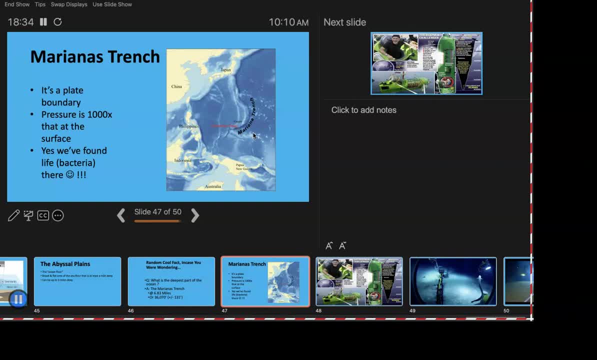 when I was growing up. the Pacific Islands. Okay, It's out that way. Java, if you've heard of that, You know we're over in that neck of the woods. We had an opportunity to see this. We had an opportunity to see this. 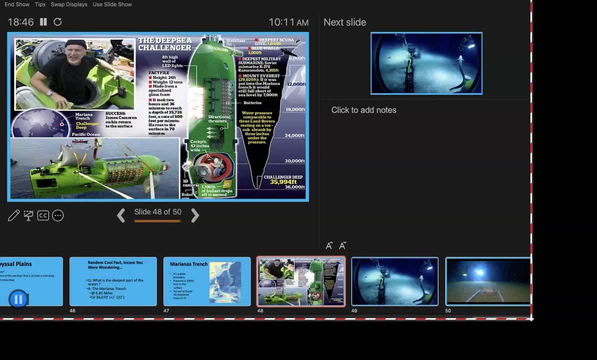 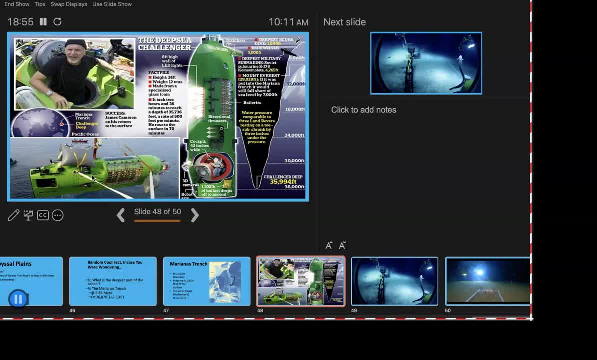 helped fund this thing And this was a really neat adventure And they learned a lot of important things. He was smart enough just not to send himself down in his family. He actually brought some scientists with him, So we could actually do some good. 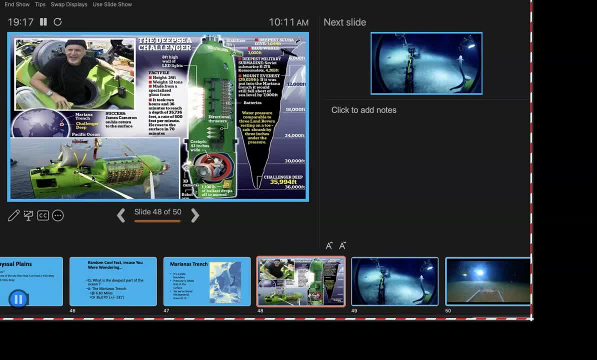 They released it as an IMAX movie and a handful of other things. Yes, sir, No. no, that was a shabby knockoff. No, apparently they did know going in that they'd been having troubles all along, But I think it imploded technically even worse. 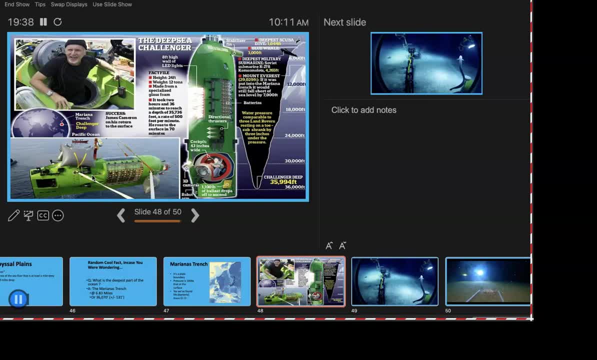 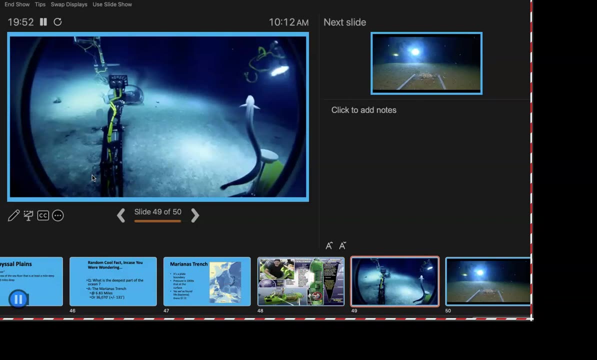 But either way it's not good. But no, this thing came down and went down, came back up. He might have even taken it back down, But yeah, Yeah, no, this one worked out okay And things are a little warped because of the lens. 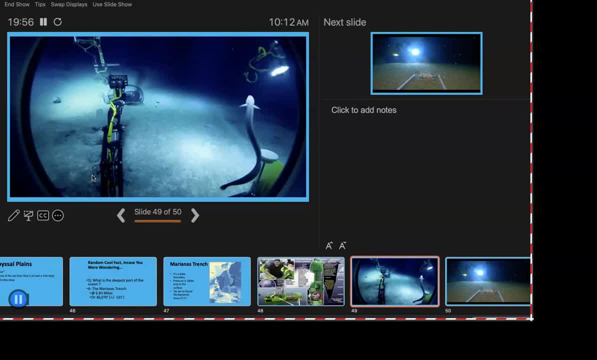 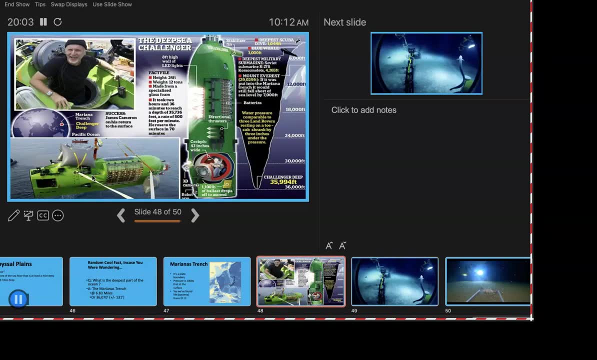 But I'm sure that fish isn't quite that long. But we saw some really neat stuff And, like I said, if you ever find the footage, Yeah, well, I'm sure it's an eel kind of thing. I'm trying to remember what the movie was called. 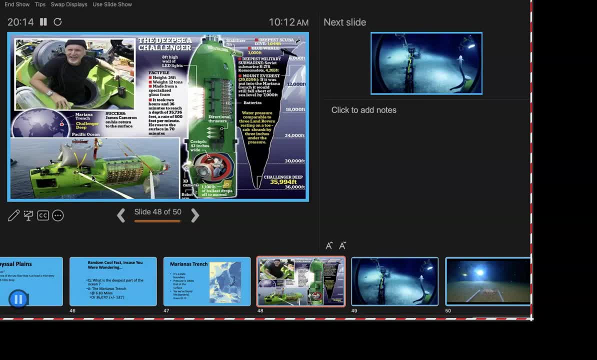 But Challenger Deep would probably be a good start If you ever want to Google it. So what we got here is a neat little thing here. So deepest scuba diving: 1,000 feet. Blue whales go down to 3,000 feet. Military submarines down to 4,265 feet. Apparently the Soviets held that record. Mount Everest, if you were to turn it upside down, would go down to 29,000 feet. So to go down to 35,900 is way farther than anyone's ever been. 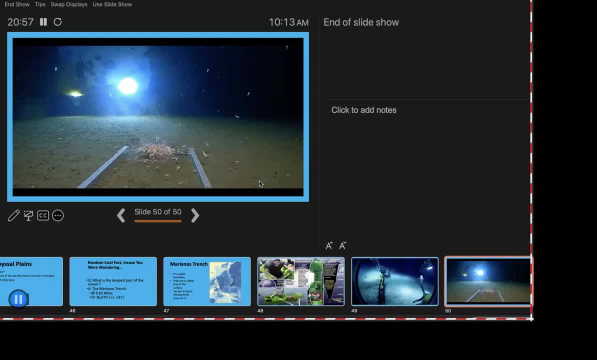 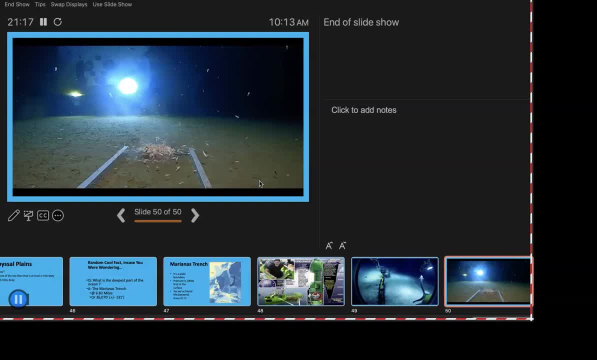 They eat sulfur, They eat sulfur, They eat sulfur, And then we work our way up the food chain. I think that's easy to believe. The hardest thing to figure out is how those critters got there in the first place, But really amazing stuff. 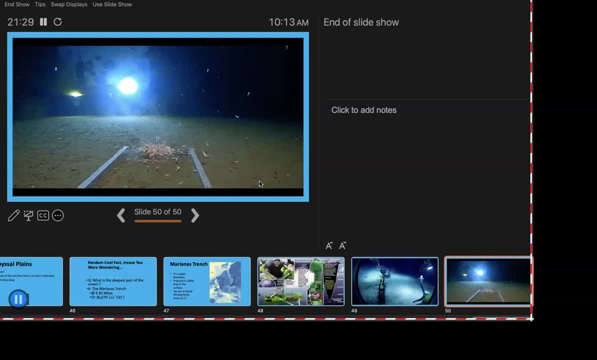 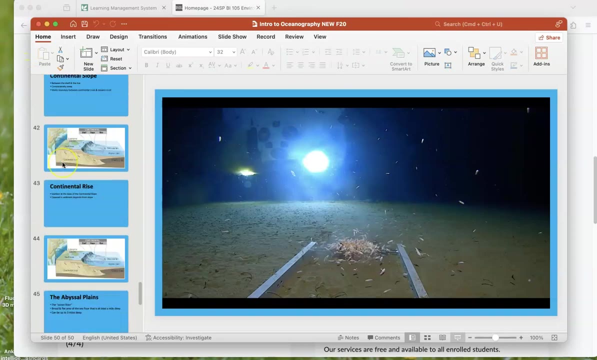 And again, if you're ever bored someday, Google this stuff, because it's some crazy things that you've probably never seen, All right. So, like I said, I just wanted to run back through that with you guys just to reiterate some of the things that we've talked about. 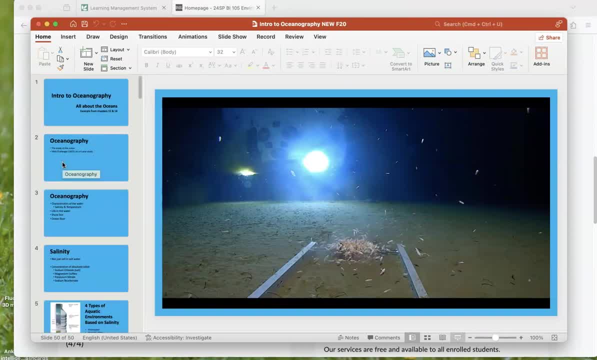 Some of the things that you see on that. you saw on 6.2,. all right that otherwise wouldn't Just want to make sure you got them. So just to reiterate then, we've got a lot of content. Many of you came in after I started this. 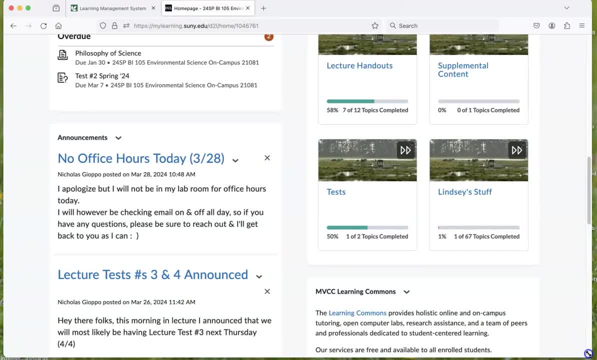 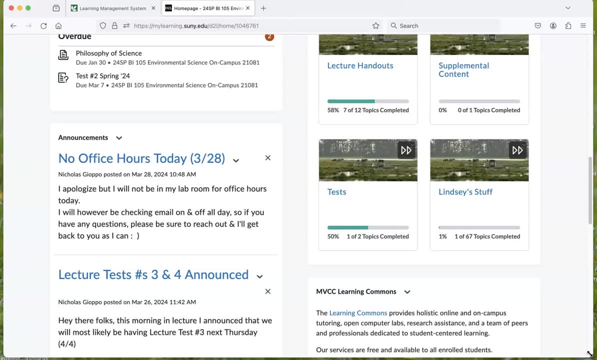 A lot of conversation, a lot of content coming from the terrestrial ecosystems handout and a good chunk of it also coming from the aquatic. all right, But there is a little bit interspersed from the straight out oceanography and very little bit from 4.2.. 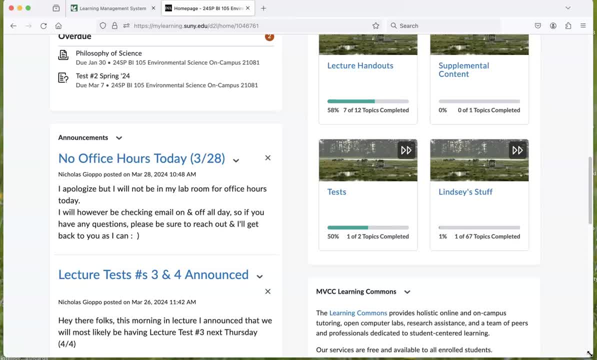 And you'll have to re-watch the watch the beginning of the class's video to find out what we're pulling out of, But you'll have to re-watch the beginning of 4.2. So I won't bore the folks that were here with hearing that again. 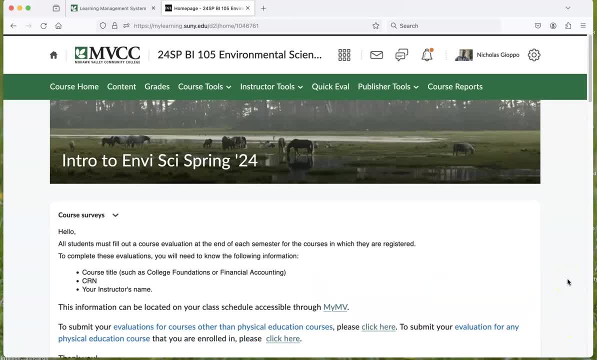 So the test. as always, I will be sitting here. If you want the pleasure of my company while you're taking it or, more so, the ability to ask me questions, please bring a laptop or tablet to campus to take the test on Thursday. 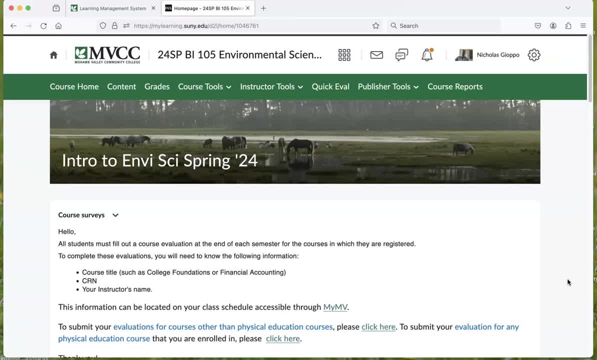 Otherwise, be sure to check the announcements To make sure that you take it. it's only going to be open a couple hours. Remember, this is meant to simulate taking the test on campus during class time. You don't get 24 hours to take this test. 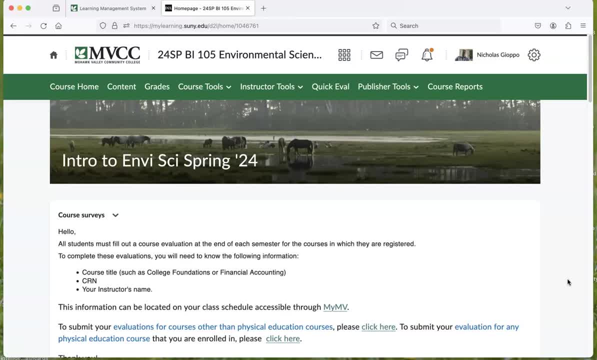 I think I left it open until noon or 1 the last time, and I will do exactly that again. So please again make sure that you check the announcements And I'll see you next time. Bye, Bye, Bye, Bye. 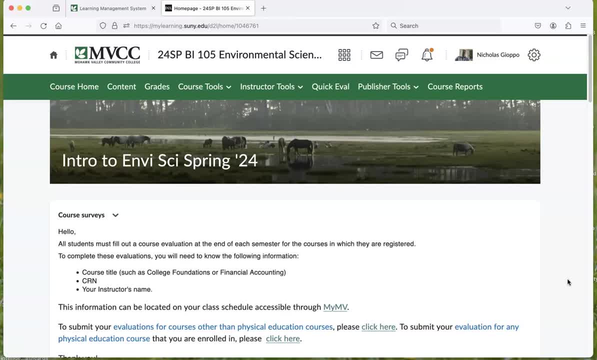 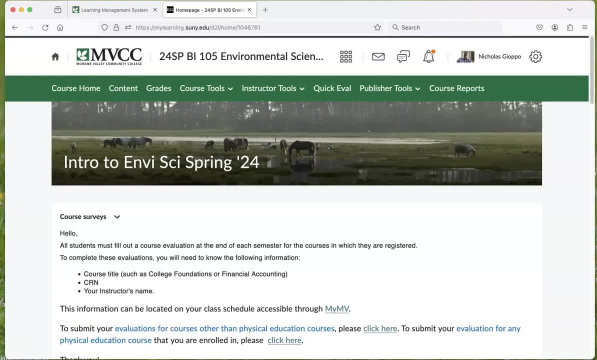 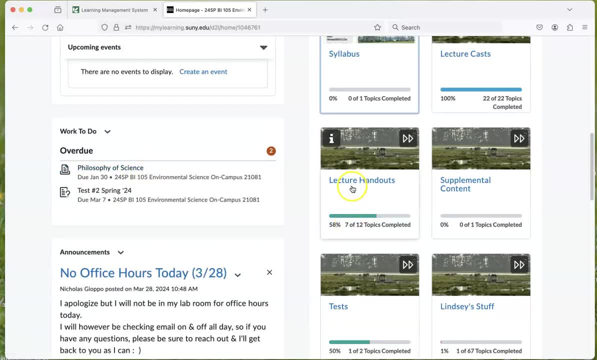 No, Awesome, Alright, Those handouts. Well, actually I will leave this open so I'm able to put the OCRI manual here. Oh, yes, Okay, so you could pull up surveys and make becomes slides. I think you're 41 out of 12.. 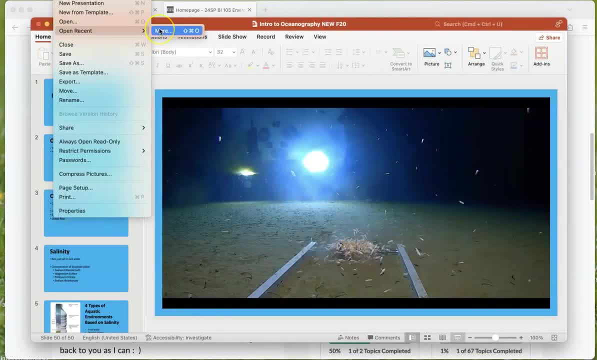 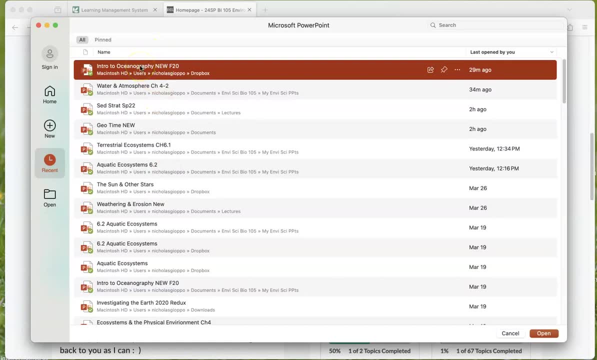 Ocean's one's on there Again. I was going to say I feel bad for letting you go so soon, but you guys chose to. you guys came late, so you're not really. will you quit interrupting me? I don't. do you want more stuff on the test? 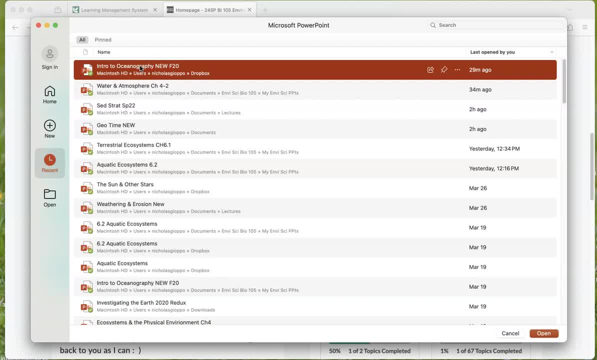 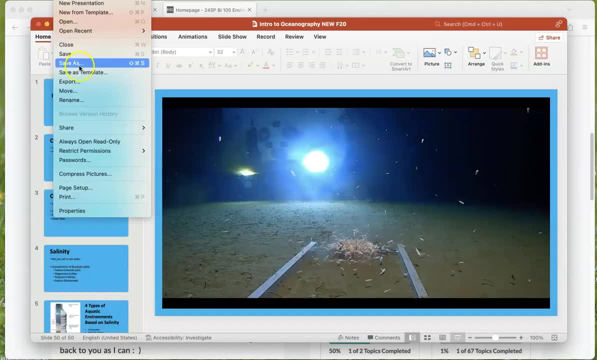 I could go over another PowerPoint if you want. All right, So, but yeah, so that's the alternative. But yeah, that was rhetorical. I didn't expect you to say yes. I hoped you didn't say yes. They hoped you didn't say yes. 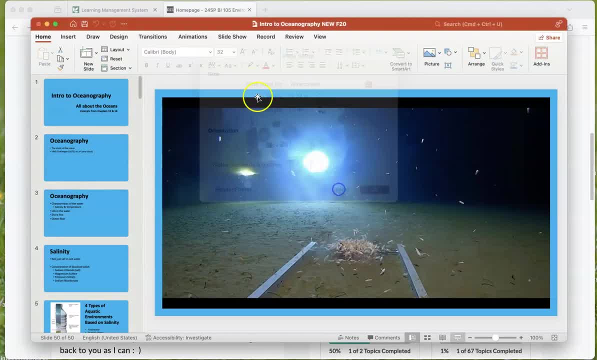 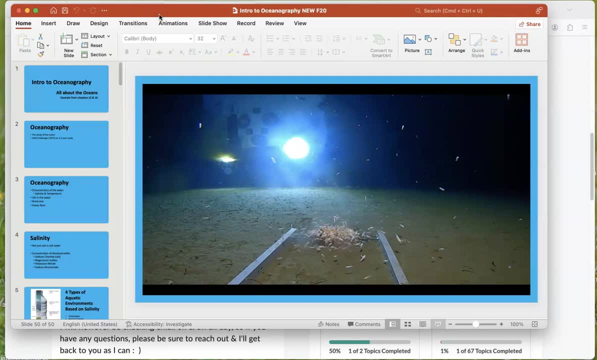 But so yeah, that's the end of the content. I don't like to cover content that won't be on the test. that you guys sort of do, inadvertently or not, But you know, you shut off your brains at a test. 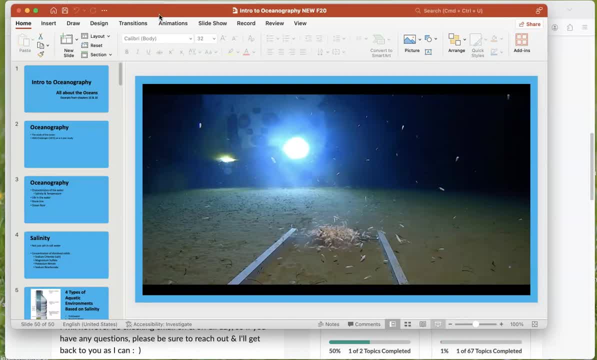 and then everything from there. we got you trained sort of going, these little cycles you know. So Everything that'll be on test four, then it'll be from you know test three to so on and so forth. So, yeah, we're going to leave it at that. 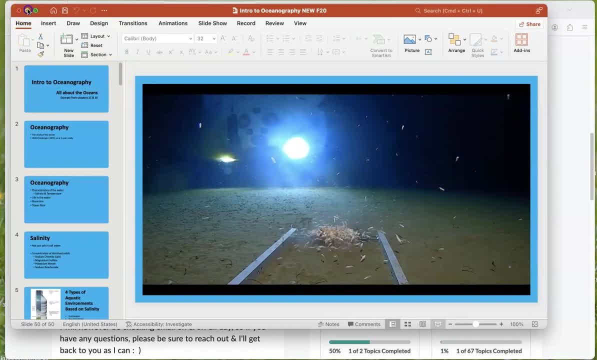 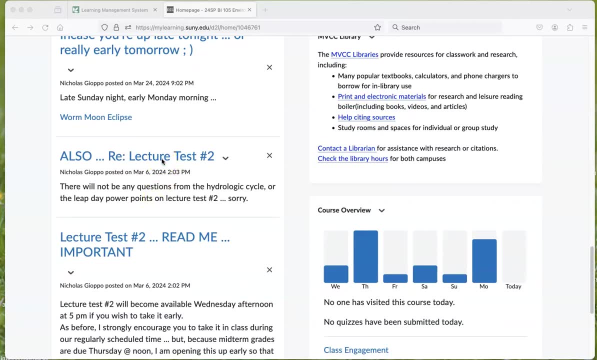 Oh, that being said, there was crumbs. We got to throw that hydrologic cycle on there Because I did not put that on the last one. So hydrologic cycle which has its own handout. Let's make sure that's there. 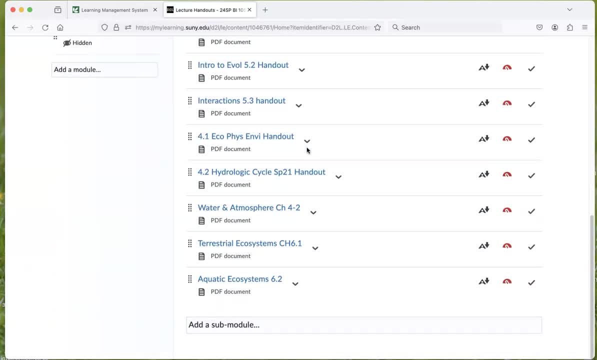 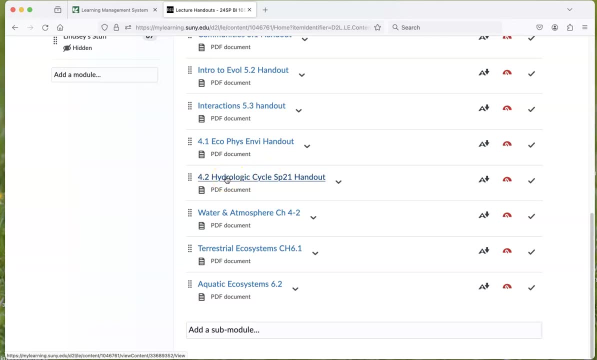 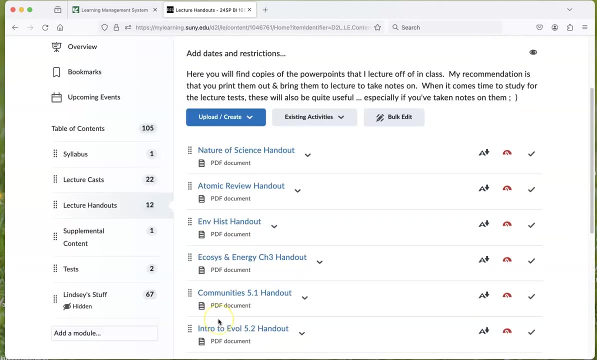 Come on Internet, Yeah. So starts right there with 4.2. Hydrologic cycle, water and atmosphere, 4.2. Terrestrial ecosystems, aquatic ecosystems And, as I said, I will post the. let's just do it right now here. 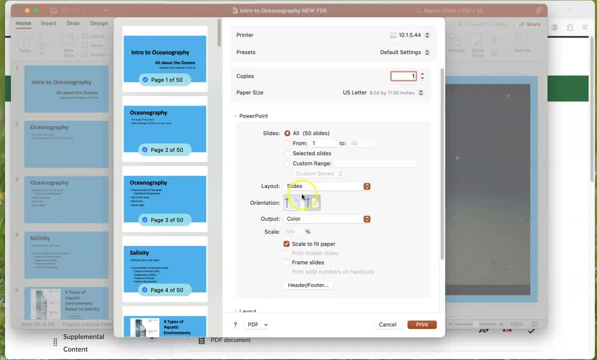 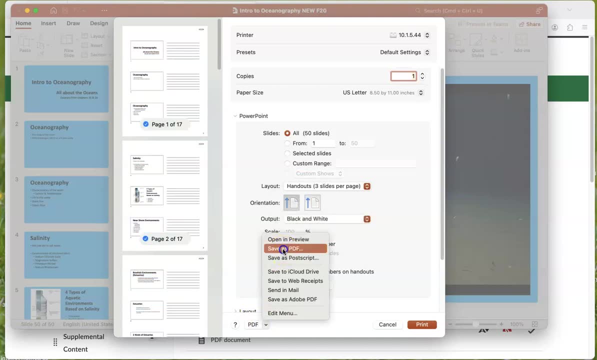 And then we'll come back. So these are the two. So these are the two. So you can click on the second one And then you'll go ahead and start by entering the information that just came in. All right? 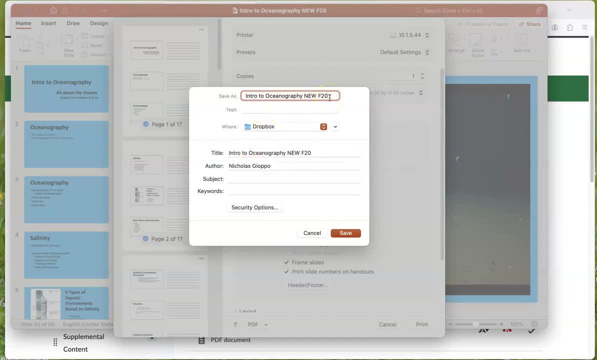 And so that's it. So there's your information. So you can go ahead and type that in there right now. And you can type it in there right now. Yeah, And you can see the data. So you can start by typing in there. 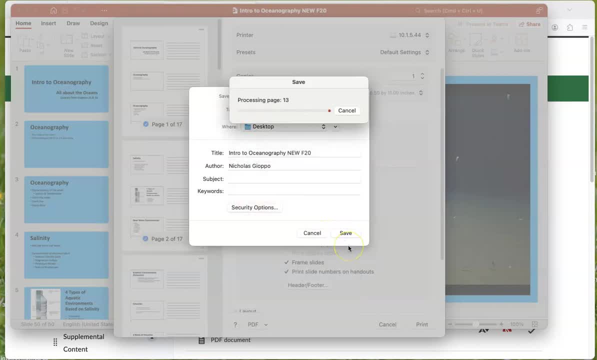 So you could put that there. So the second one: All right. So so I'll just say that there's the two. You can type that in there. So, except for the two. So if you don't know, I'll be getting that. 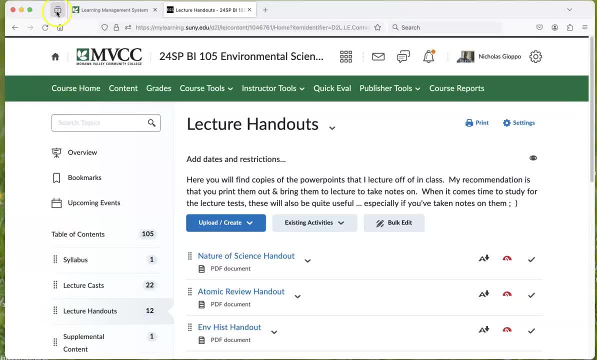 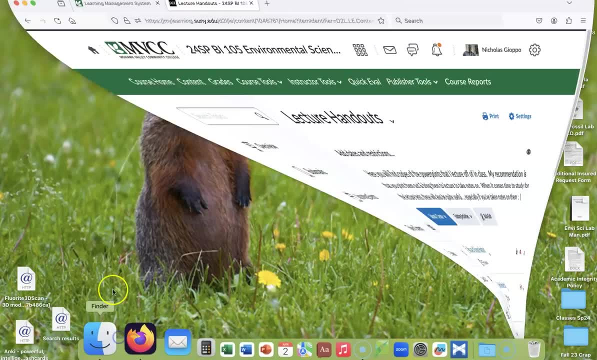 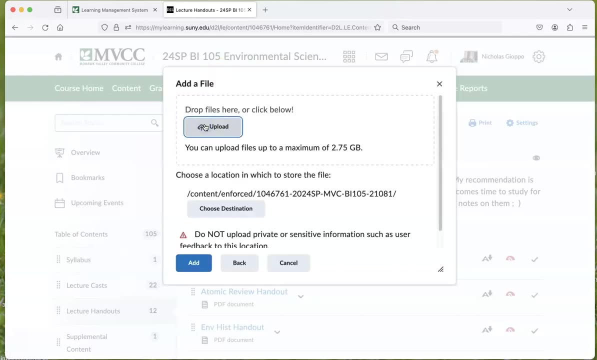 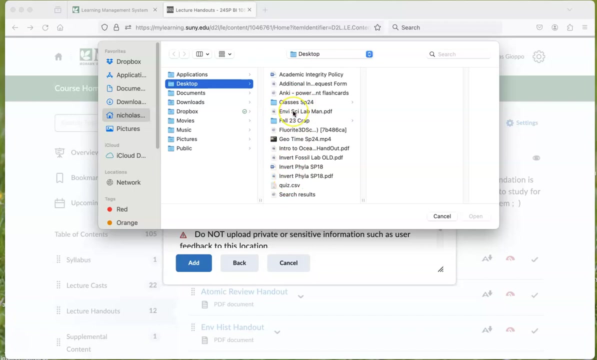 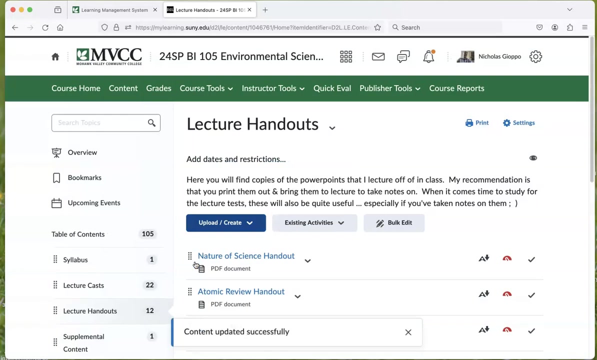 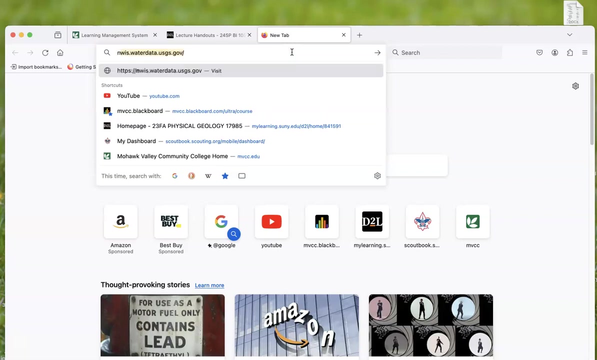 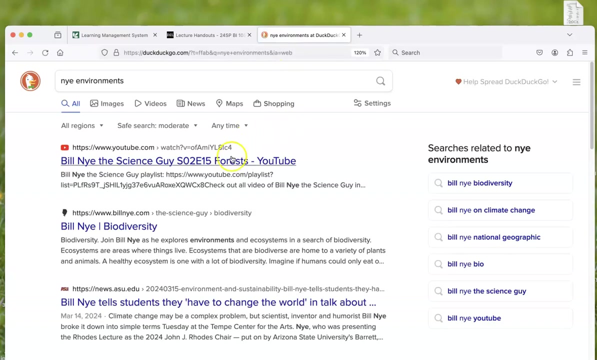 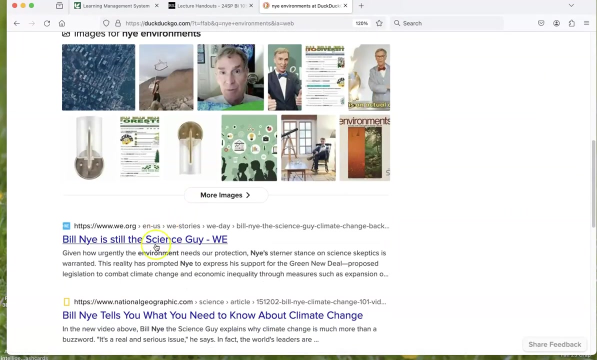 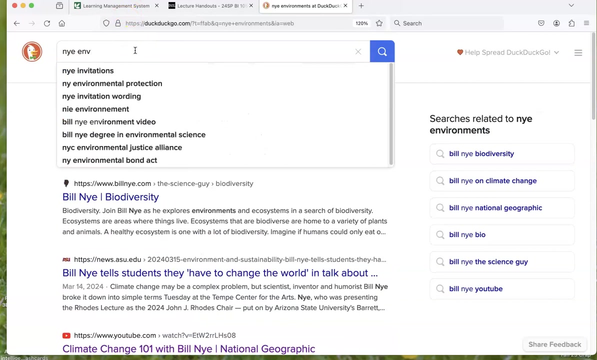 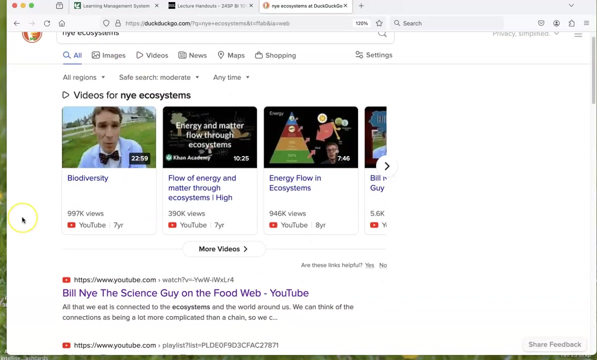 Okay, So we'll stop there. There it goes, Alright, and actually there's one more thing we want to run through here just for a minute. I thought he had an environment swap Ecosystems- Better than some rando on YouTube. 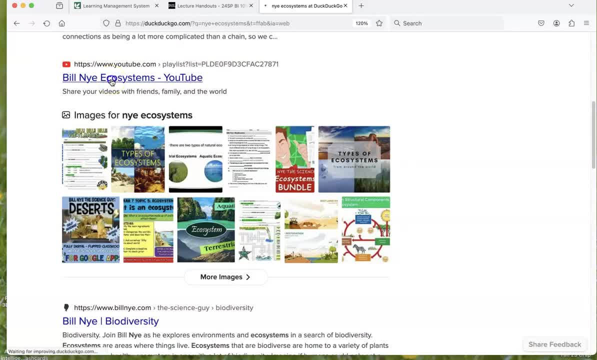 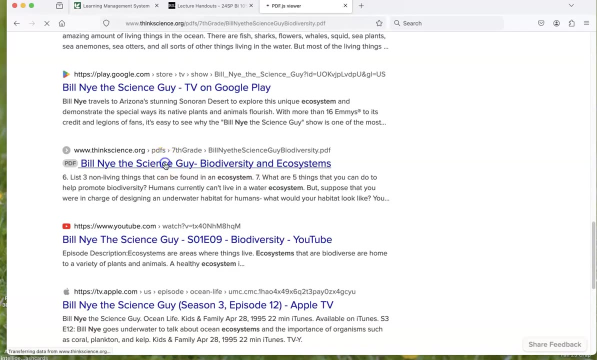 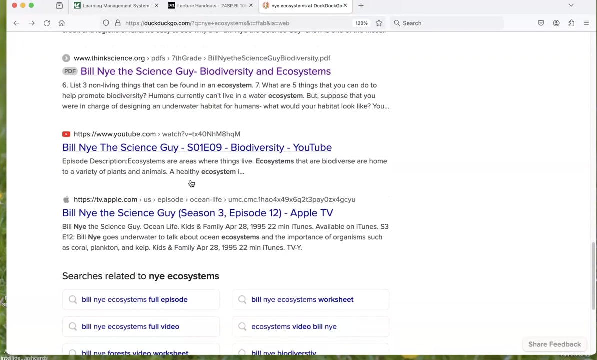 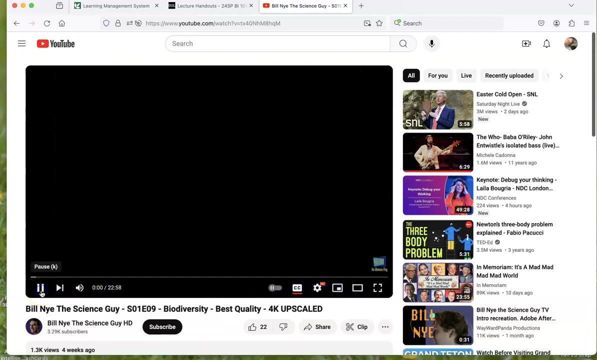 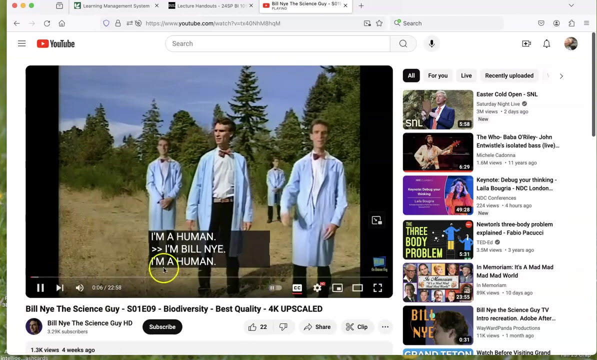 Okay, Yeah, there is one, it's just not. I thought there was one. Maybe it's just under the biodiversity. Okay, Oh, I feel like I'm a human. I feel like I'm a human. I'm a human too. 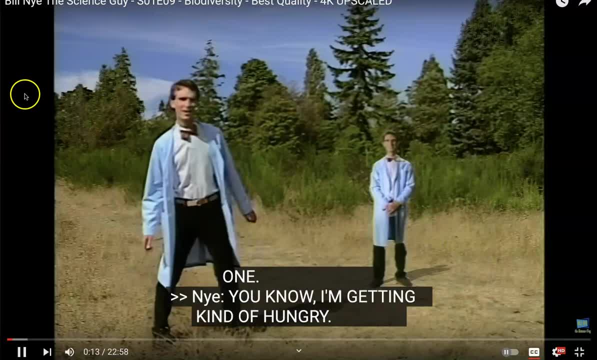 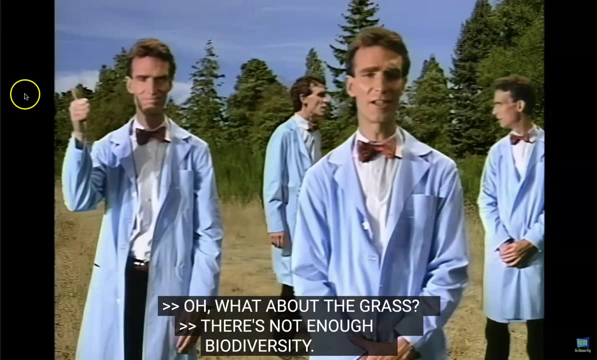 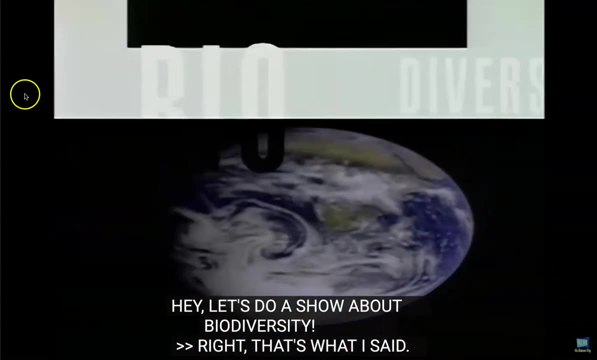 Are we the only species around here? No, but we're the dominant ones. I don't see any other species. Where's the grass University? Okay, Okay, Okay.